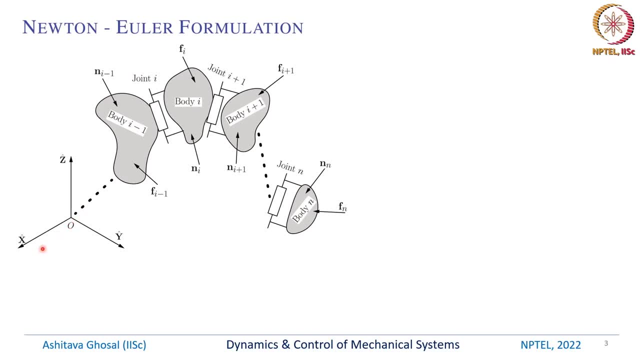 which starts from rigid body 0, which is fixed to x, y and z. so this is the reference coordinate system. the first rigid body is fixed to this fixed base or the fixed reference coordinate system. in between any two rigid bodies we have a joint, so between i minus 1 and rigid body i. 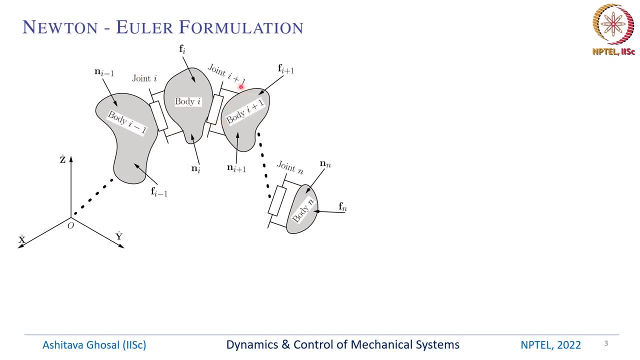 we have a joint i. likewise, there is a joint i plus 1 between rigid body i and i plus 1. okay, and we also assume that this is rigid body i minus 1. there is an external force, f i minus 1 which is acting on this. similarly, there can be a external moment and i minus 1 which is acting on. 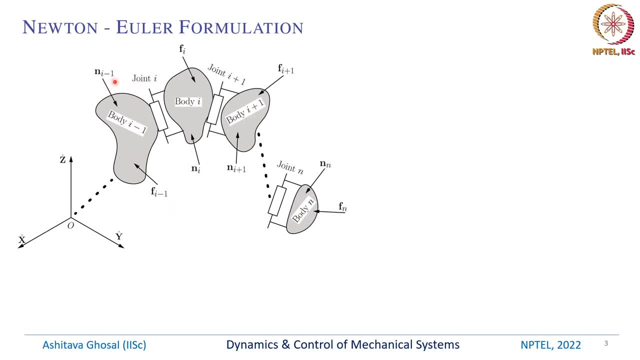 this rigid body i minus 1. so these are vectors. you okay, three by one vectors. likewise for rigid body i. we have a moment in i and a force, f, i, which is acting. so in this schematic of a serial chain, one end is fixed, one end is free, as i mentioned. 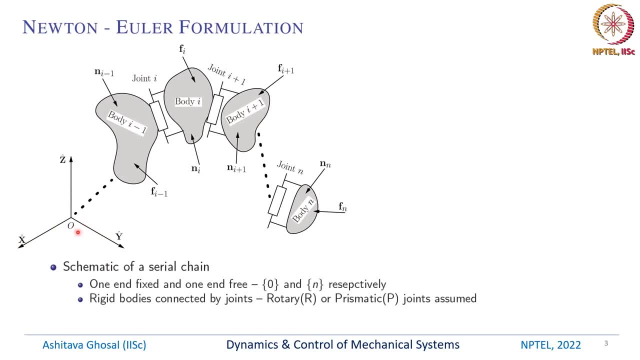 the fixed end is with this x, y, z coordinate system. the last rigid body is the nth rigid body. it is shown by this curly bracket n, and these rigid bodies are connected by joints. so in the newton euler formulation we will assume that the joints are rotary or prismatic joints. so rotary allows rotation. 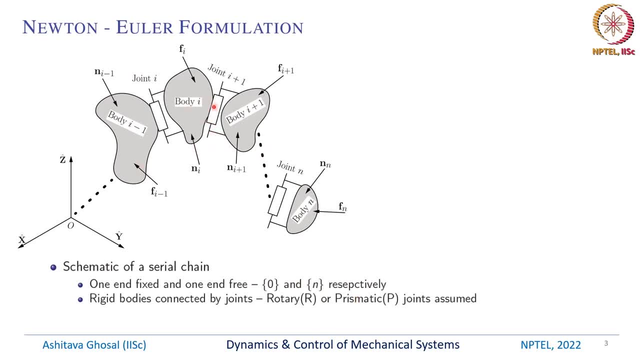 between two connected rigid bodies and prismatic joint allows relative translation between the two connected rigid bodies. the force f, i and moment n, i acts on the rigid body i, as I've mentioned, and we will look at the free- die, free body diagram of rigid body i. 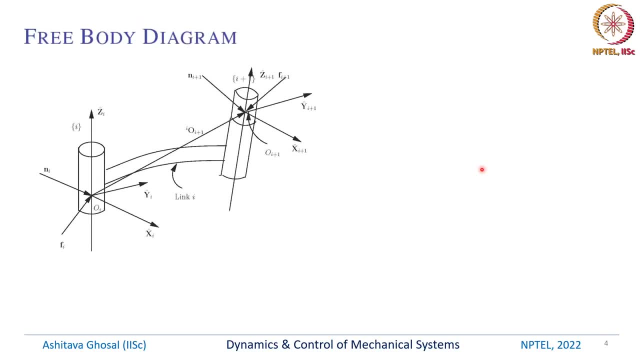 so in this example schematic, I am showing you one rigid body which is link i, one end there is one joint and the other end there is another joint. so between two rigid bodies there is joint, or at the two ends of a single rigid body there are two joints. both mean the same thing and we will 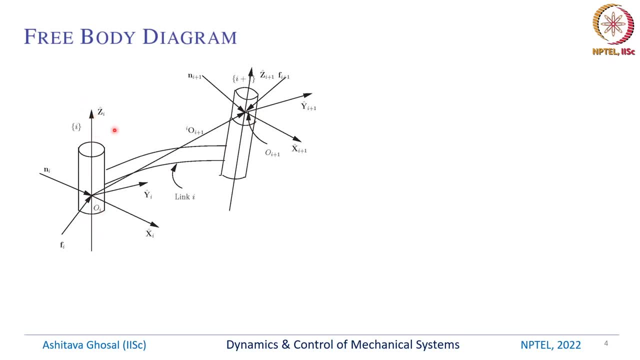 assume that the rotary joint is here or a translatory joint is on this joint, and then this z? i axis is along the joint axis. so x- i is one coordinates axis, y i is the other and z? i is along the joint axis. and we have this force, fi and ni, which is acting at this oi, the origin of the ith coordinate system. 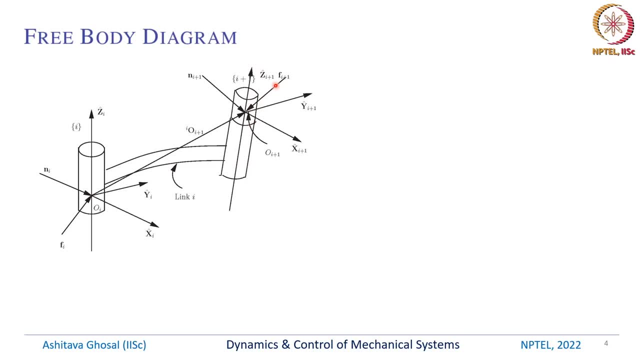 likewise, we have a joint axis z, i plus one. okay, this is the rigid body. i plus one is after this joint. and then we also have forces fi plus one and moment ni plus one, which is acting at the origin of the i plus one at coordinate system. 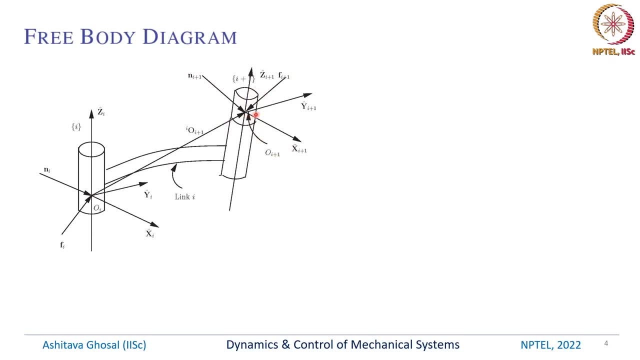 so this is oi plus one. the origin of the i plus one coordinate system is located with respect to the ith coordinate system by this vector, oi plus one. okay, so this is a vector from one origin to the next origin, and again we have one x axis, a y axis and a z axis for the rigid body: i plus one. 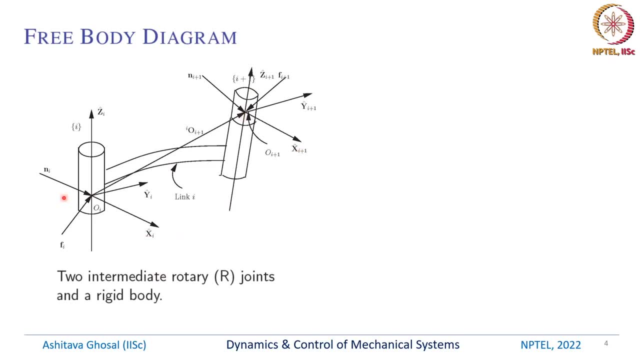 so in this example we are showing the two intermediary rotary joints. these joints could have been also translatory joints and, as i mentioned, fi and ni denote the forces and moments exerted on rigid body. i by link, i minus one, so the i minus one link is before this. 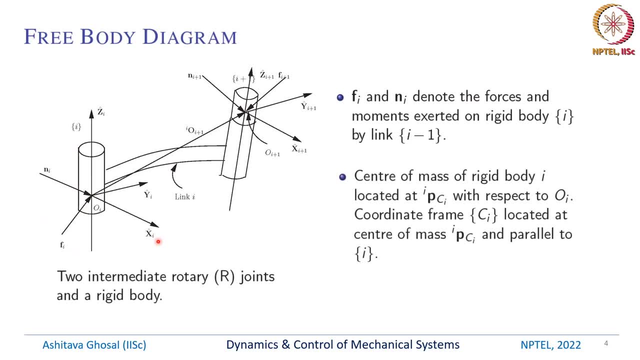 joint, the center of mass of rigid body. i is located at some with, at some vector i, pci, with respect to oi. so some point here, the quad, a coordinate system, is attached to the center of mass, which is denoted by ci. it is located at the center of mass and it is parallel to x, i, y, i, z, i. so basically we take this: 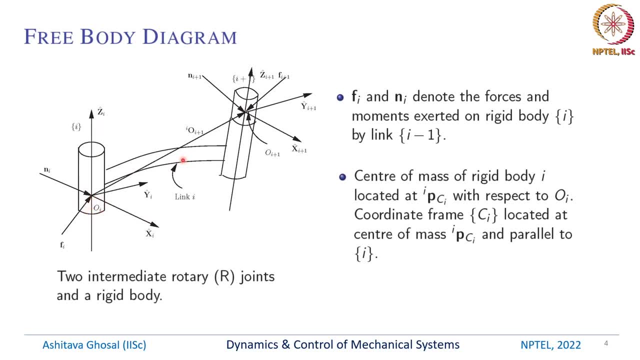 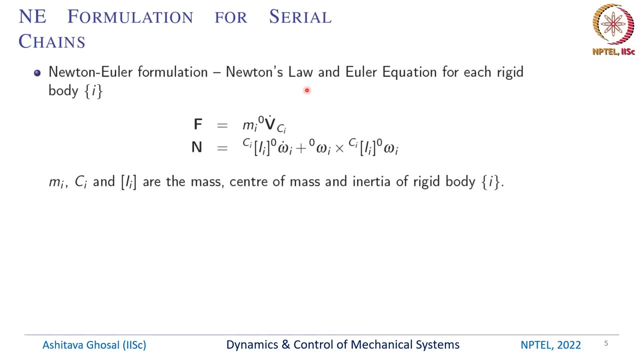 coordinate system x, i, y, i, z, i with y and shift it in a parallel way to the center of mass. so the newton- euler formulation goes like this: we apply newton's law and euler's equation for each rigid body. i- and the newton's law is given by force- is mass times. 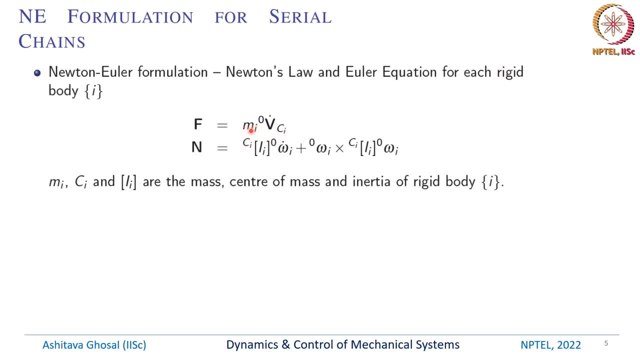 acceleration. so mi is the mass of the ith rigid body, f is the external force. i dot is the acceleration of the center of mass of the ith rigid body with respect to the zero coordinate system or the reference coordinate system. likewise, the moment, external moment, n can be written as some i into alpha, which is zero omega. i dot into omega, cross i omega. 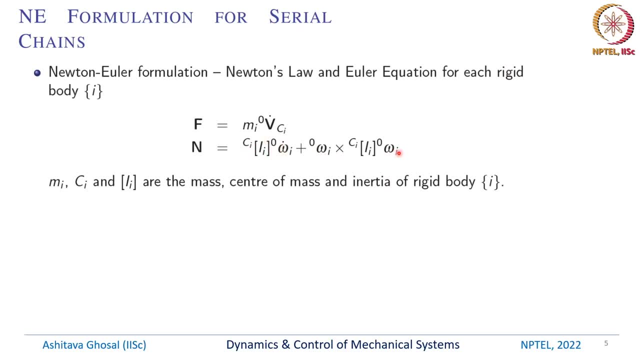 and in both of these you can see that the acceleration and the angular velocity they are with respect to the zero coordinate system or the fixed reference coordinate system, and the inertia is with respect to the center of mass, which is what the ci is showing with respect to a coordinate system which is also fixed at the center of mass. 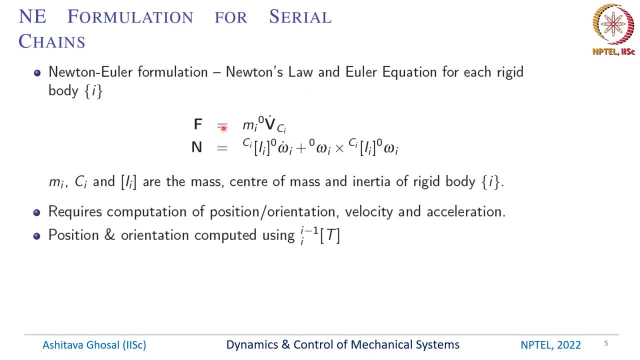 so, in order to use these right equations, or we want to substitute what is acceleration and angular velocity and angular acceleration, we have to start from position and orientation, then we have to go to velocity of each link and then we have to go to acceleration of each link to obtain the position and orientation of any link. 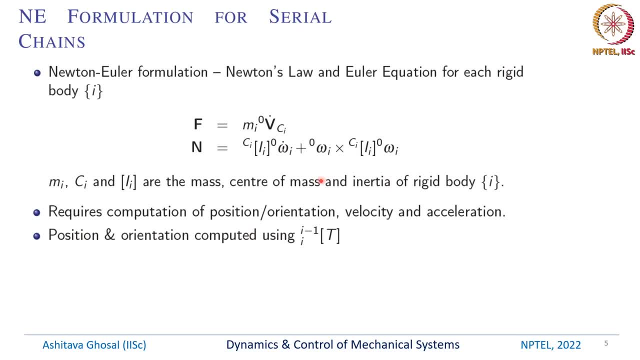 with respect to the zero or the fixed reference coordinate system. we go back and use this 4 by 4 homogeneous transformation matrix. okay, we had discussed this. so this homogeneous transformation matrix, the top 3 by 3, contains the orientation of rigid body i with respect to i minus 1 and the 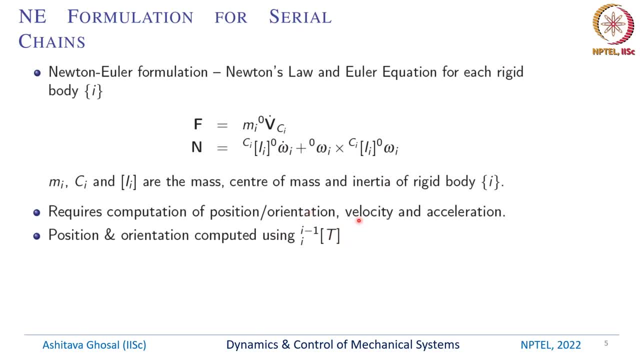 last column, the 3 by 1 vector contains the position of the coordinate system attached to rigid body i with respect to the rigid body i minus 1. okay, so this we can obtain. the linear and angular velocity can be computed, computed using propagation formula. this was also discussed. 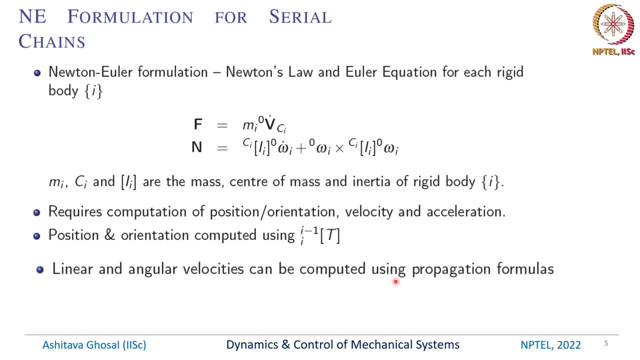 last week. so basically what we have is we start with the fixed base, which we know- zero velocity and zero angular velocity, okay, and then we go to the next link and if there is a rotary joint, then theta dot is added, if it is a prismatic joint, then the linear velocity is changed. 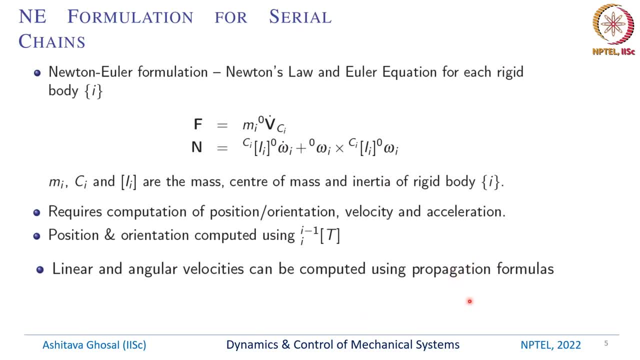 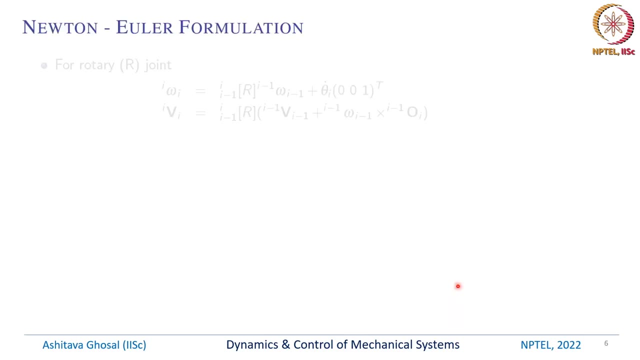 with di dot. so we had derived this propagation formulas. starting from a fixed base, we could find the linear and angular velocity of each link. okay, as we go along the chain, so we will use those propagation formulas. so just to recapitulate, for a rotary joint, the propagation formula: 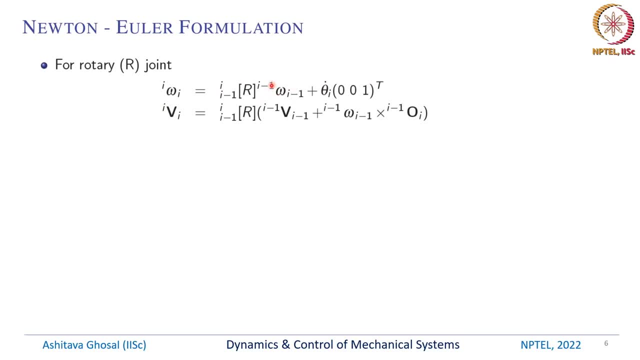 was the following: so if you have the angular velocity of i minus 1, we can find the angular velocity of the next rigid body with respect to its own coordinate system. then we can find the angular velocity of the ith rigid body, the next rigid body, in its own coordinate system. by this formula it tells you that we have to pre-multiply. 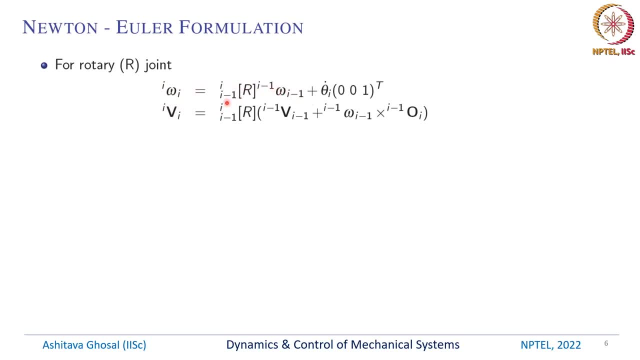 this angular velocity with the rotation matrix i to i minus 1, and then we have to add this rotate angular velocity at the rotary joint, which is theta dot zero zero one. remember the joint axis is along the z-axis, so hence it is theta dot zero zero one. the linear velocity. 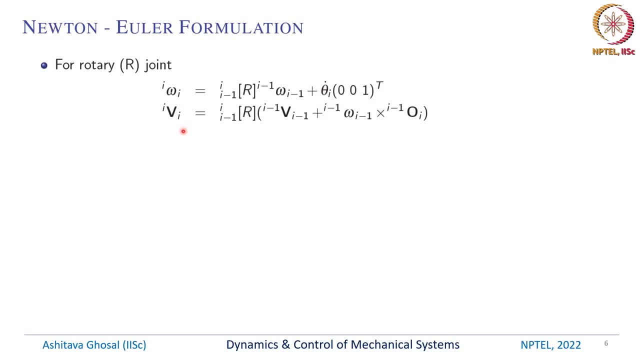 of the origin of the ith coordinate system or the linear velocity of the point at in the rigid body. i, at the origin of the coordinate system, is again the linear velocity of the i minus 1th rigid body plus some omega cross r. okay, so i minus 1 o i located at the origin. 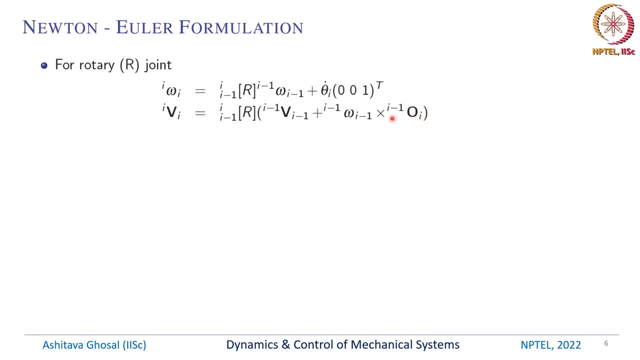 of the next rigid body with respect to the previous rigid body, the origin of the coordinate system attached to the previous rigid body and this is the angular velocity and, again in order, the propagation formula we pre-multiplied by some rotation matrix, so it looks like this iterative form. okay, so what we will do is we will put some i equals, let's say one which 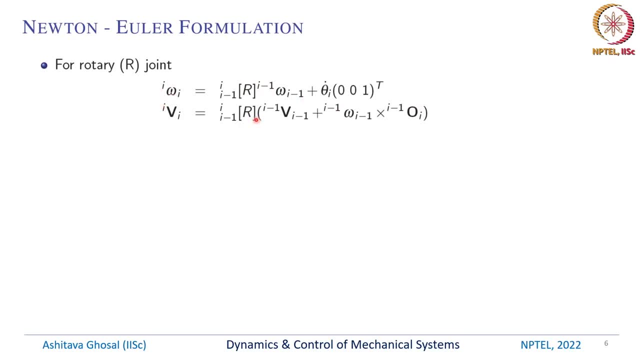 will be zero, omega zero, and we find out one, omega one. similarly, i equals zero will give me one v one, and so on. then i equals two, then three, and so on all the way to the last rigid body, n. so for prismatic joint we have omega is same. so the previous link, i, omega, i minus one will. 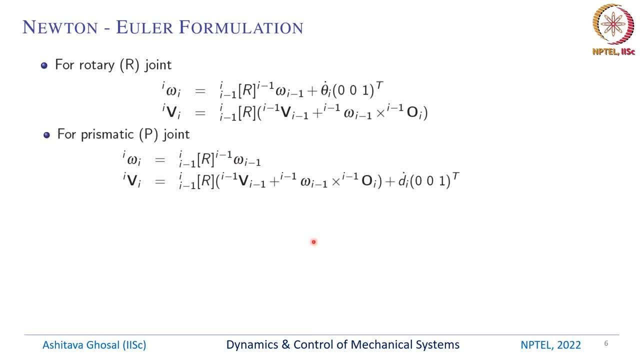 be same as the i, omega, i of the next link, because the prismatic joint does not allow it, only allows relative translation, which is what is shown here: the linear velocity of the next link. the origin of the next link will be the linear velocity of the origin. 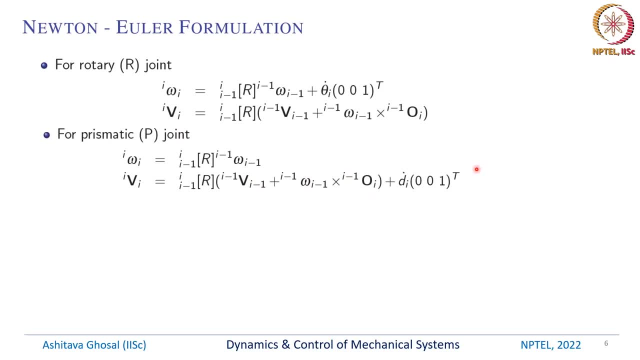 of the previous link, plus some omega cross r, plus what is happening at the translatory joint, or the prismatic joint, which is d, dot, zero, zero, one. and again the joint axis is along the z axis, so that is why we have this zero, zero one, the acceleration of an arbitrary point on the rigid body. i we can differentiate the. 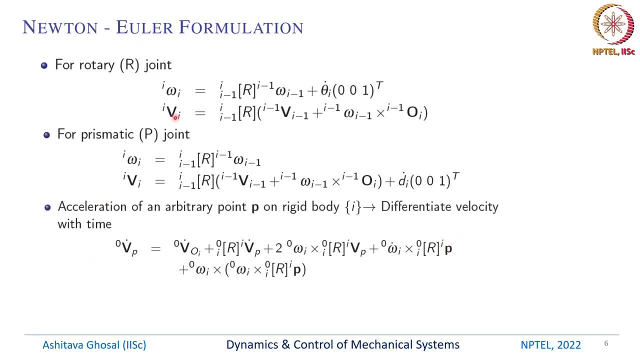 velocity with respect to time. so if it were a rotary joint, we could differentiate this and then what we will see is that the velocity of this point p, when you differentiate and you will get acceleration of this point p, it is nothing but the acceleration of the origin plus the relative acceleration, plus some two omega. 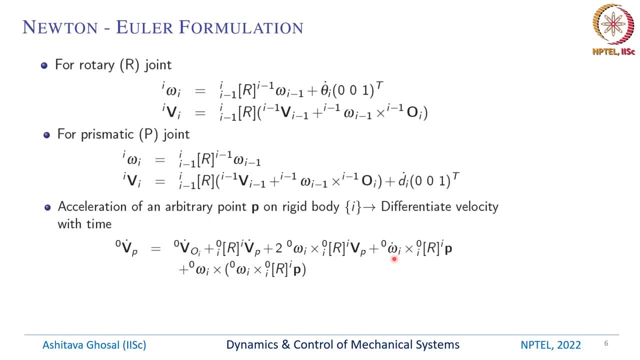 cross V, relative plus alpha cross R, and then omega cross, omega cross R. So we had looked at this equation earlier. So these are the five terms typically in the acceleration of a point in a rigid body which is both translating and rotating with respect to a previous fixed 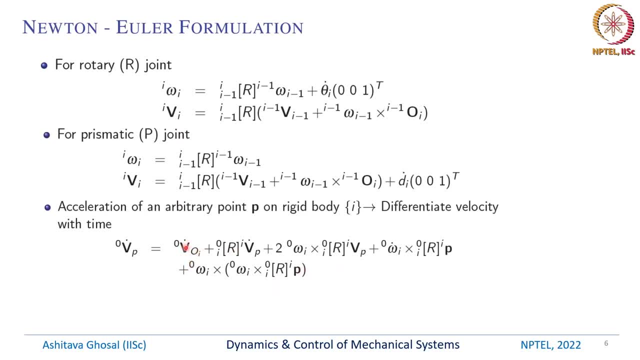 reference. So this we have seen. This is the acceleration of the origin. This is like similar to the AND problem we have discussed earlier. This is the relative acceleration of the AND. Then this is the two omega cross: V rel, which is the Coriolis term. This is: 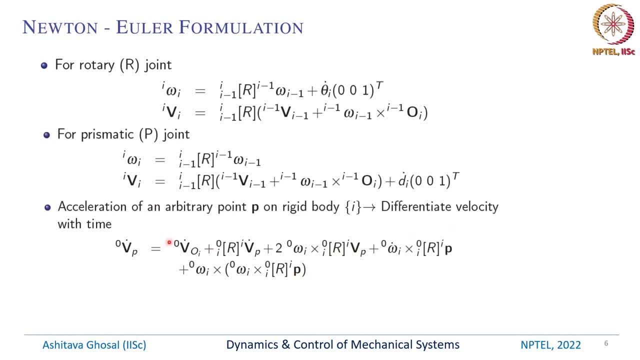 the tangential acceleration and this is the centripetal acceleration. So we can obtain this. We have seen it earlier. All we are doing it, we are writing it in a formal way. If the point on the ith rigid body is stationary or this IP vector is constant, then there. 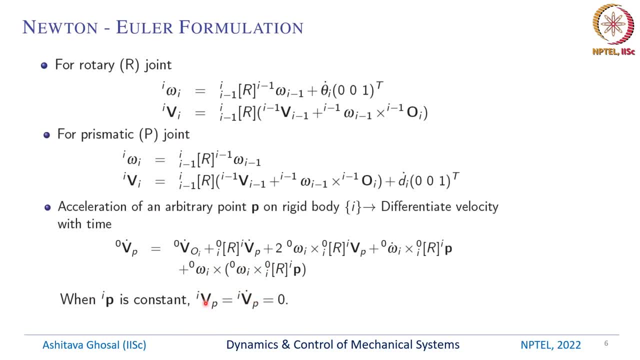 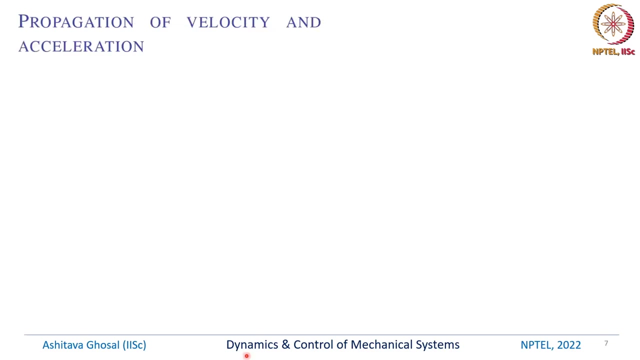 is no relative acceleration or relative velocity. So we have both these terms, which is this relative acceleration term and this Coriolis term zero. So we will only have the acceleration of the origin plus some alpha cross R And then this centripetal term. So continue with this idea of propagation of velocity. 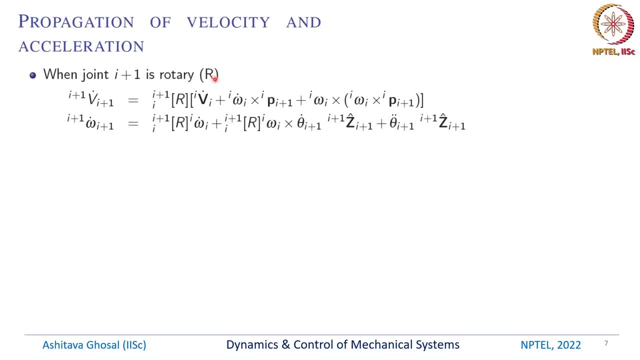 and acceleration. If the joint I plus 1 is a rotary joint which allows relative rotation between the two rigid bodies, then the acceleration of the I plus 1th rigid body written in its own coordinate system will have three terms: Okay, Rotary joint. there is no relative velocity. 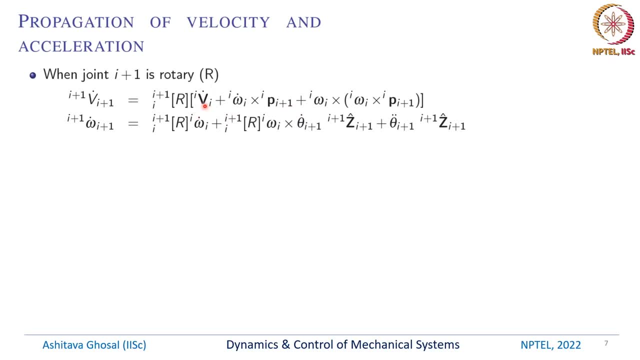 or relative acceleration. So we have the acceleration of the origin plus alpha times R. plus this centripetal term, The angular acceleration of the I plus 1th link is again nothing but the angular acceleration of the previous link. Then what is happening at the? 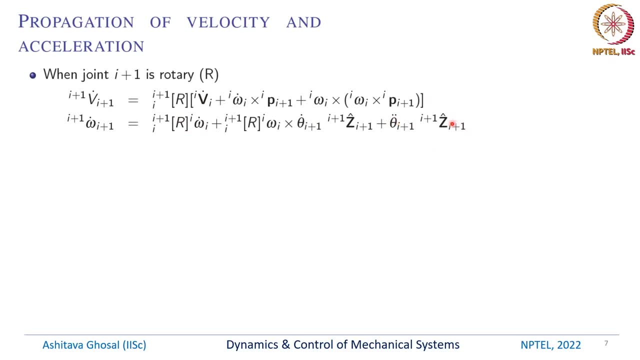 joint, which is theta I plus 1 double dot along the z axis. but interestingly we will also have one additional term. Okay, i omega i cross theta i plus 1 dot. okay, and this is also along the z axis. so it turns out. 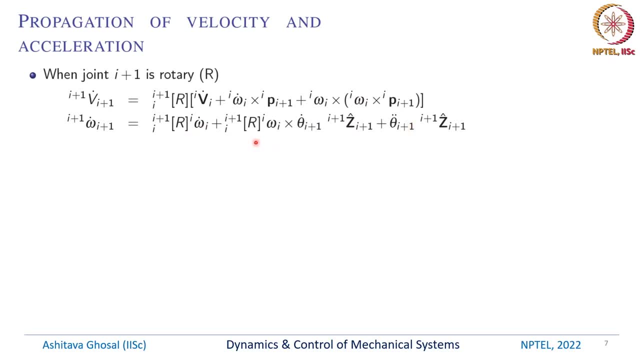 that we will get alpha and then theta double dot plus something like omega cross theta dot. okay, so this is what appears when the joint i plus 1 is rotary, and all of these can be derived from first principles. if you are interested, when joint i plus 1 is prismatic, we'll look at the 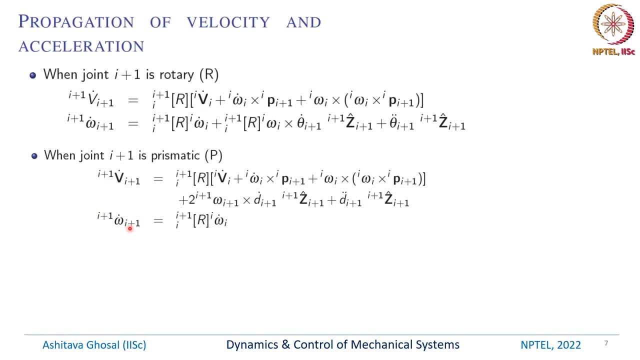 simple case first, which is that the acceleration of the angular acceleration of the i plus 1th link is same as the angular acceleration of the ith link. okay, because there is only relative translation between the two links. however, the linear acceleration of the i plus 1th, 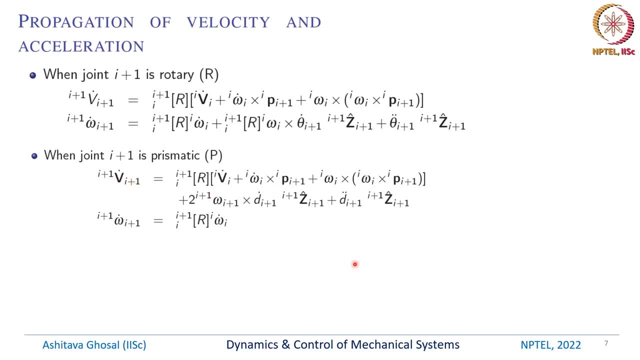 rigid body will now have all the, the linear acceleration of the i plus 1th rigid body will now have all the five terms which are there in the expression for acceleration. so we have the acceleration of the origin, then alpha times r. this is the tangential acceleration, this is the centripetal term. 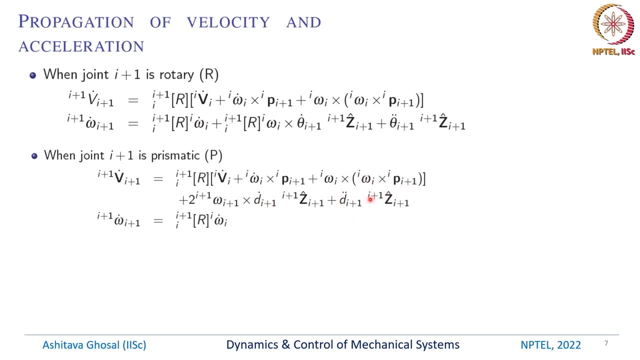 then this is the coriolis term and this is the term which is showing the relative acceleration of the point in its di plus 1 double dot. okay, so we have this generic expressions for propagating both the linear velocity, the angular velocity, the linear acceleration and the angular acceleration from one link to the next link. 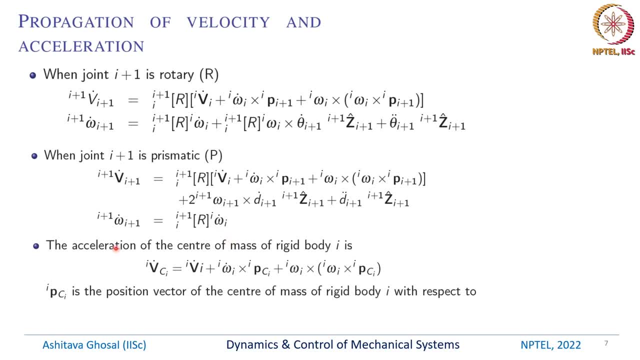 the acceleration of the center of mass is nothing but the acceleration of the origin plus alpha times, r plus the centripetal term. okay, so we will need the acceleration of the center of mass because we have the centripetal term and we will need the acceleration of the. 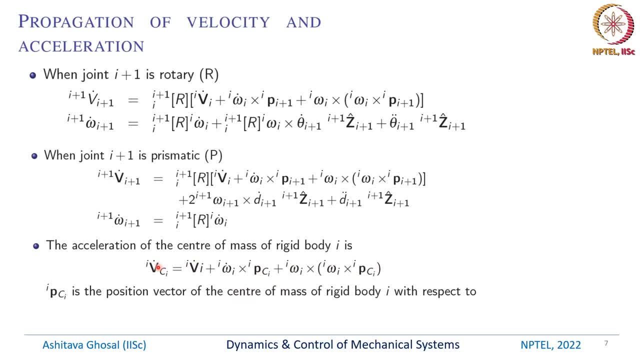 origin plus alpha times, r plus the centripetal term, and we would like to apply newton's law, which is: f equals mass times, the acceleration of the center of mass. so the acceleration of the center of mass of any link can be obtained by the acceleration of the origin plus alpha times, the distance from the origin to 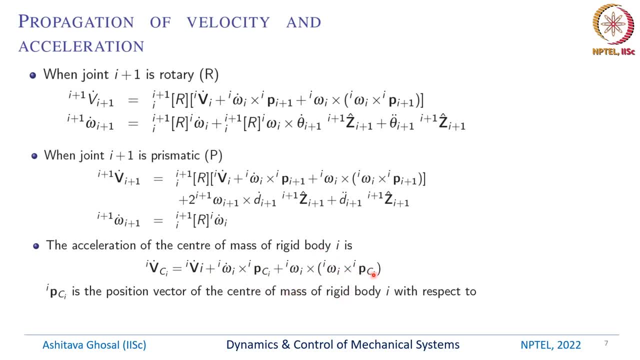 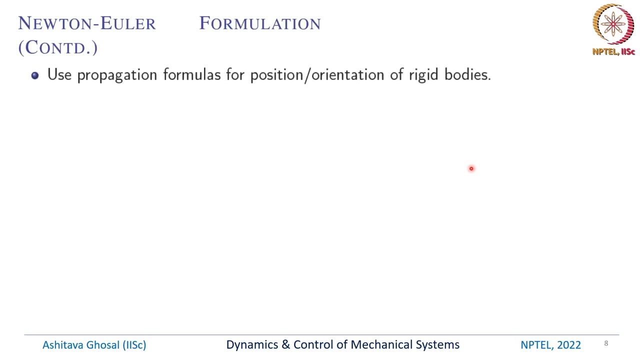 the center of mass, plus omega cross, omega cross r. okay, so i p, c, i is the position vector of the center of mass of rigid body, i with respect to the origin oi. So let us continue with this Newton Euler formulation. We have the propagation formulas. 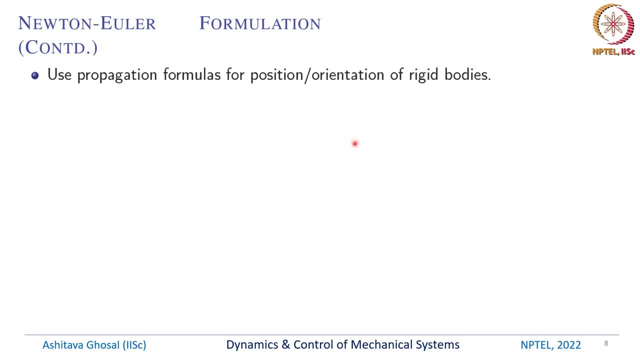 for position and orientation of rigid body, basically using 4 by 4 homogeneous transformation matrices, and then we need the outward iterations for velocities and acceleration, which is given in this algorithmic form. So we start from I equals 0 and we end at n minus 1, because 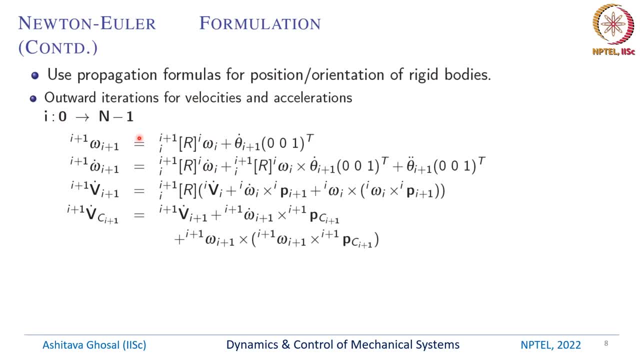 for n minus 1,, the left hand side will give the nth linear and angular velocities and acceleration. So what do we have? And this is for rotary joint. We are showing you these examples. We need to change these formulas if there is a prismatic joint in between. but 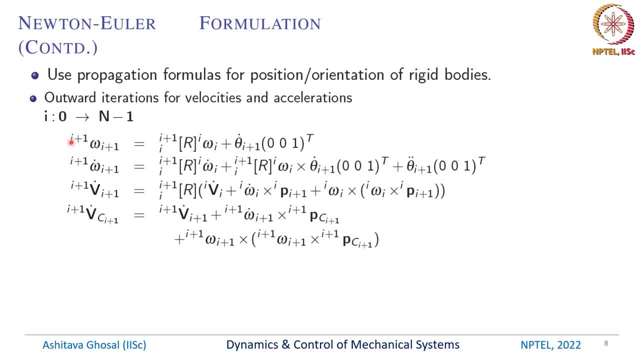 nevertheless, the angular velocity of the I, The I plus 1th link, can be written in terms of the angular velocity of the Ith link plus the rotation or angular rate at the rotary joint. The angular acceleration of the I plus 1th link can be written in terms of the angular acceleration of the Ith link, then this term. 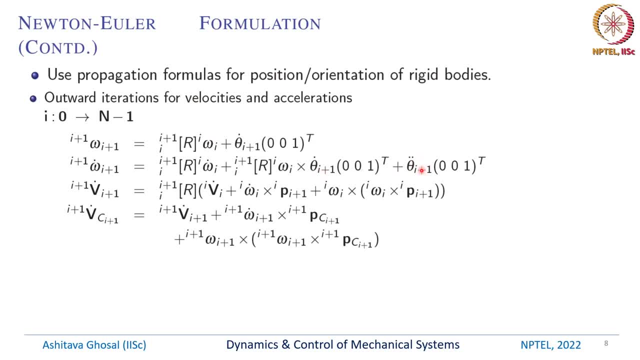 of omega cross, theta dot and then theta double dot, I plus 1.. The acceleration of the origin, of the I plus 1th link, the linear acceleration, is again three terms, which is the linear acceleration of the origin plus the tangential term, which 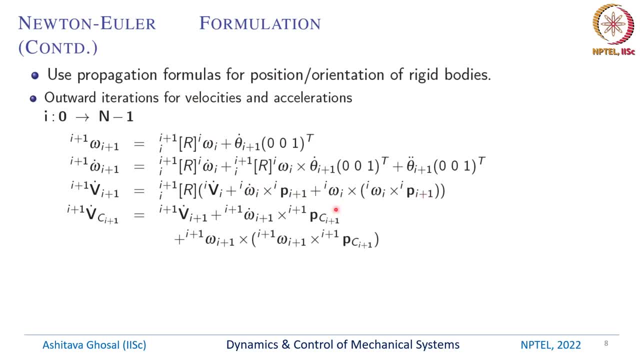 is alpha cross r, and then this is the centripetal term, The acceleration of the centre of mass of the I plus 1th link can be written in terms of the acceleration of the origin plus omega cross R, plus omega cross omega cross R. Okay, so with these formulas I can start with some. 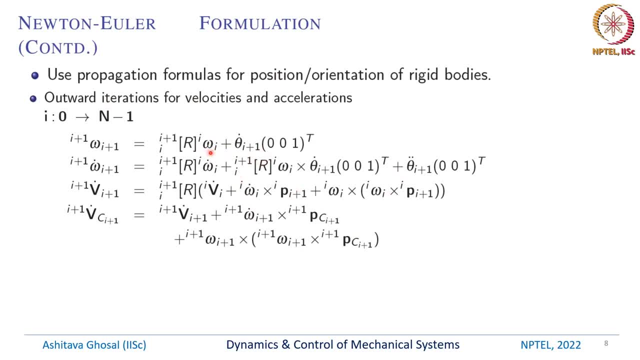 I, and if we substitute what is happening on the right-hand side, we'll get the terms in the left-hand side. Once we have this linear acceleration of the center of mass, then the angular velocity of the i-th link and alpha of the i-th link, or the angular acceleration of the 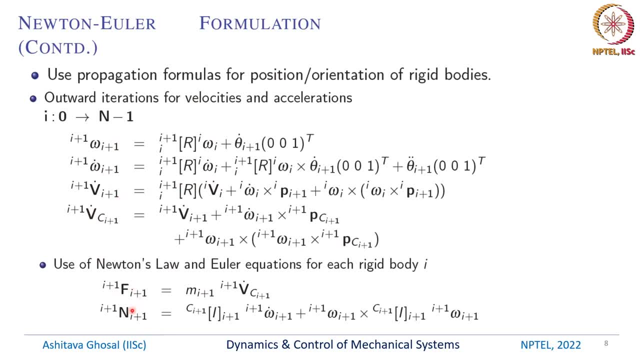 i-th link, then we can apply Newton's law. So what the Newton's law says is that the external forces is nothing but mass times acceleration. This is what is written here, and we are writing it with all this superscript and subscript because it is in the form of a outward iteration. So 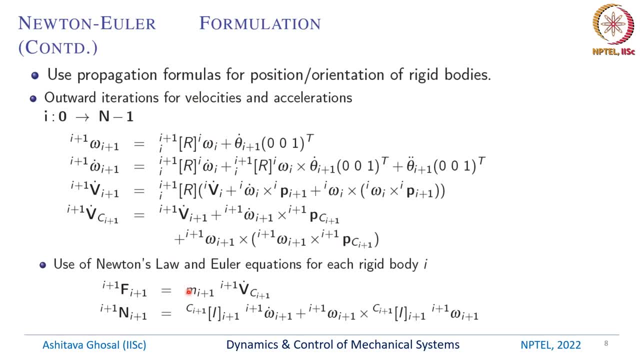 I can start with i equals 0 and end with i equals n minus 1. actually, sorry, so we end with i equals n minus 1. similarly, the external moment is nothing but i into alpha plus omega, i, omega. okay, so this is euler's equation, this is newton's law and this is euler's equation, so we can apply both of these. 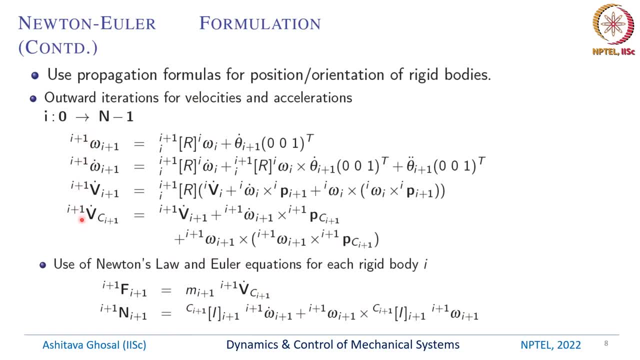 we know the right hand side because from this outward iteration i know what is omega dot, i know what is omega, i know what is the acceleration of the center of mass. so i know what is the right hand side here. we know, of course, what is the mass and what is the inertia matrix. so if i 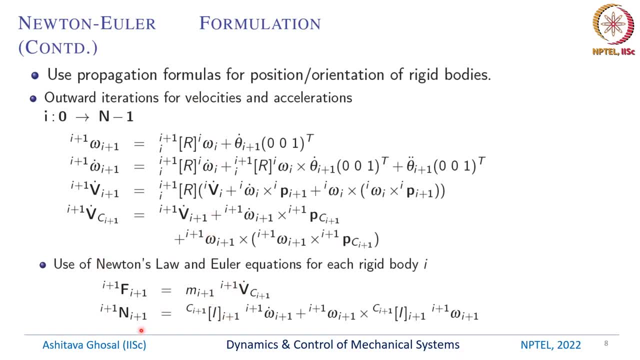 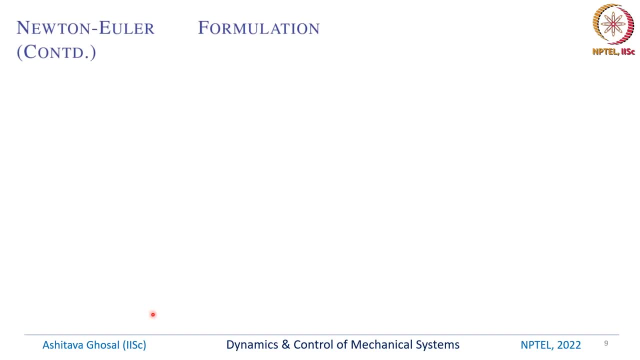 substitute all these things on the right hand side, i will get the force and the moment which is acting on the link. i plus one once i know what is this force and the moment which is acting on a link. this is called the outward iteration. so we start with position, then velocity, then acceleration, and then we compute the. 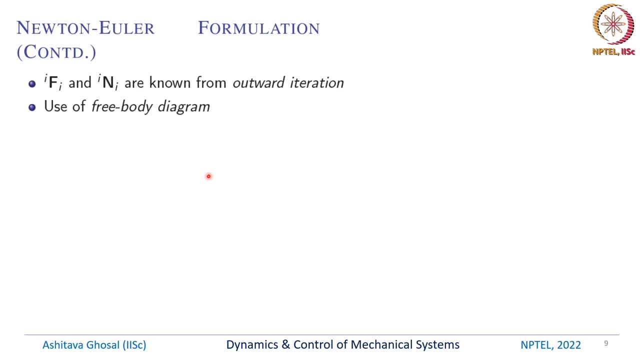 forces and moments using newton's law and using euler's equation. so we have used, basically, some kind of a free body diagram in addition to what are these propagation equations. so once we have these forces and moments which are acting on the ith link, we go backwards. okay, so 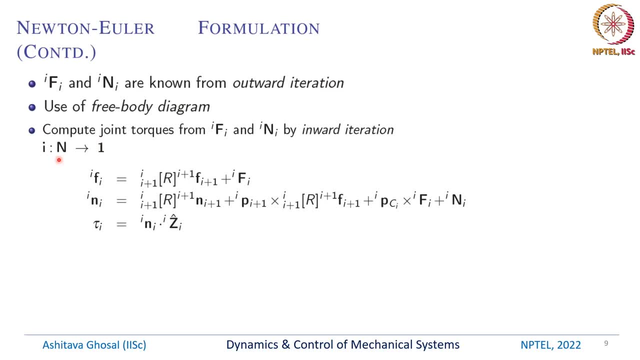 this is called inward iteration. so we start with i equals n and then we go backwards. so what is i at for nth rigid body? so the ifi will be nothing. but what is the external force which is acting on the link n plus what was the result of the force and moment which is acting on the ith link? so this is: 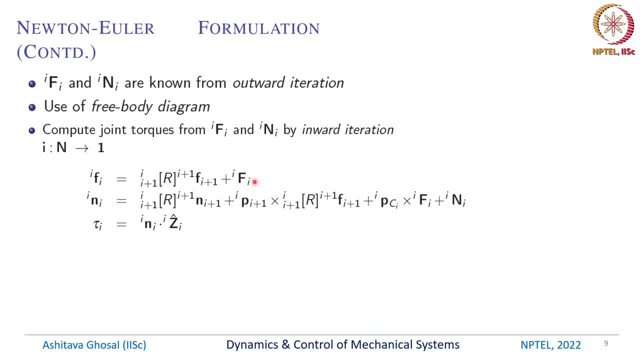 the applied force of the application of newton's law. so we have this last rigid body which is rotating and accelerating and so on. so, based on newton's law, we can find the f equals m a, so we know m a. similarly, euler's equation moment is equal to i. alpha plus omega, cross i, omega, so i. 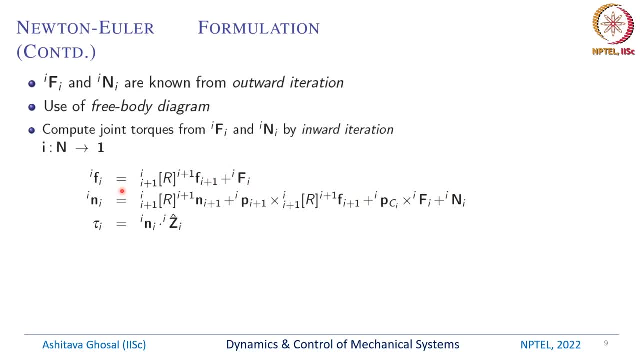 know the right hand side, which is fi and ni, and then we can find what is the external force which acting at the end. so if the robot is pushing something or if there is a some external force which is acting on the last link, then we substitute it here and then we find what is the force acting. 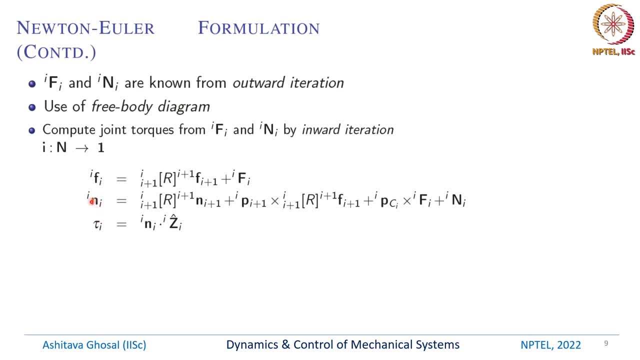 on the ith link. similarly, we find the moment which is acting on the ith link based on what is the external moment obtained from euler's equation, then the r cross f, which is the moment of this external ifi which is coming from here, from newton's law, and then we have these two terms. 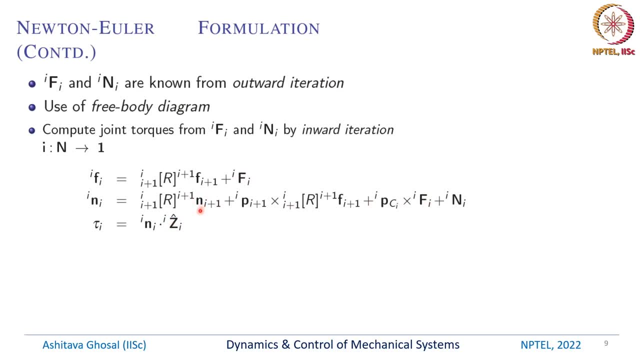 which is the external moment which may be acting on the last link and the external force which may be acting on the last link. so once we have the right hand side from the outward iteration, we can use these expressions to obtain what is the force at the moment which is acting at the origin of the ith link. okay, so for i equals n. we know what is the. 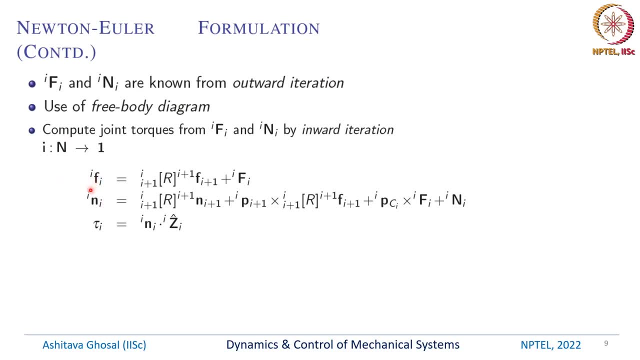 force and moment which is acting at the coordinate system which is fixed at the nth link. the last step in this newton euler formulation is to find the torque which is acting on the ith link. so the last link. there is a joint okay between the nth link and the n minus 1th link. 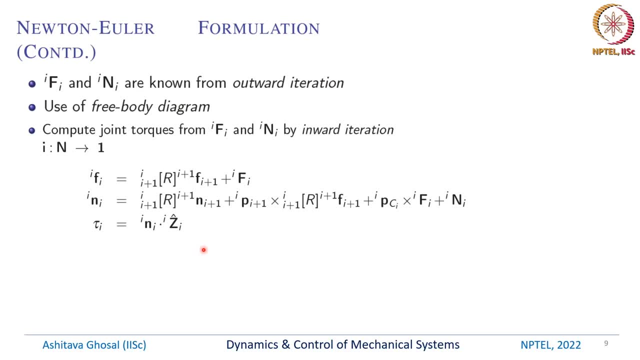 there is a joint, we assume that for the moment that that joint is a rotary joint. so if it is a rotary joint, the z component of the rotary joint is given by some motor or some torque. okay, so the torque which is acting about the z-axis is the 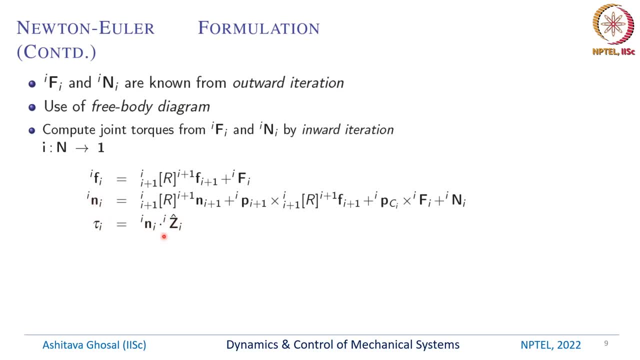 z component of this ini which we have computed. if you want to include gravity, all we need to do is we need to set the zeroth coordinate system, or the fixed coordinate system. is accelerating upwards by g? okay, so if it is accelerating upward by g, all the outward propagation formulas for acceleration. we now see this g, okay, so 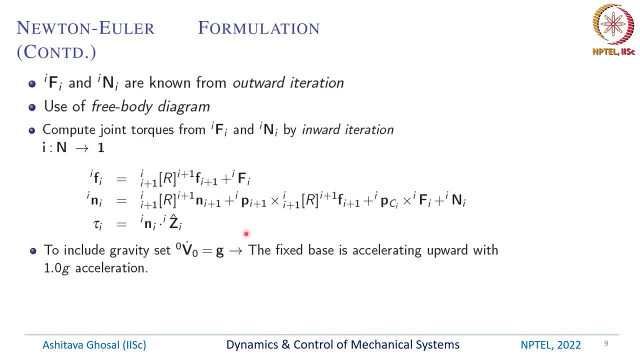 hence all the links will see the effect of gravity. so this algorithm which i showed you, that first we position velocity, then acceleration, and we go outwards, which was the outward iteration, and then we use it into newton's law, and then we use euler's equation to find this fi and ni, and then we 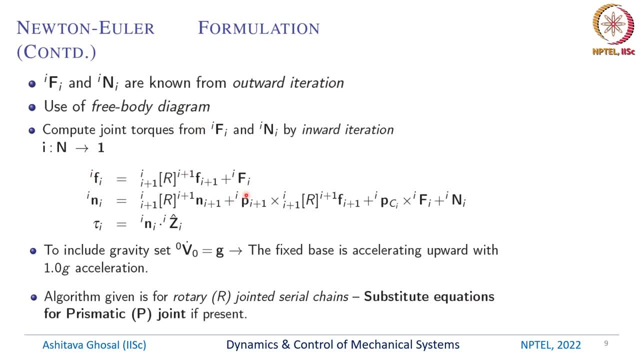 use free body diagram and we go backwards. so we find what is the net force which is acting at the origin of the Ith link and the moment which is acting at the origin of the ith link, and then we say that the torque which this rotary joint is giving by means of a motor or some other means, is the z component. 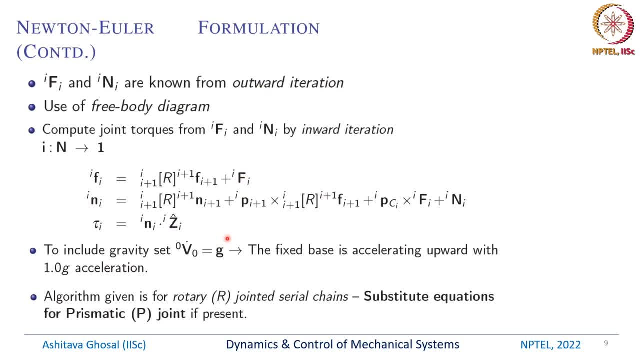 of the moment, moment. okay. So all this formula was for rotary joint. If it is a prismatic joint, we need to change these outward equations. So wherever there was velocity, we would now have di dot. Wherever there was acceleration, we would have all the five terms in the acceleration. 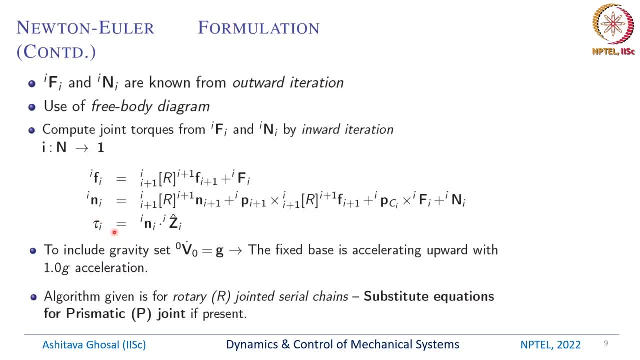 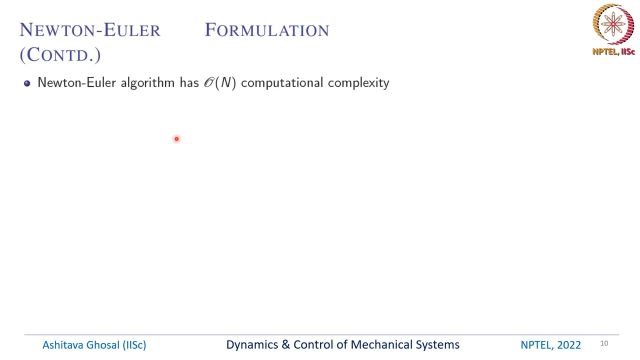 And this, instead of torque, we would have some force which is acting along the z-axis or along the z-direction. So basically, we carefully substitute the equations for a prismatic joint in both these outward iterations and inward iteration. So this Newton-Euler algorithm is very well known. It is very, very efficient. 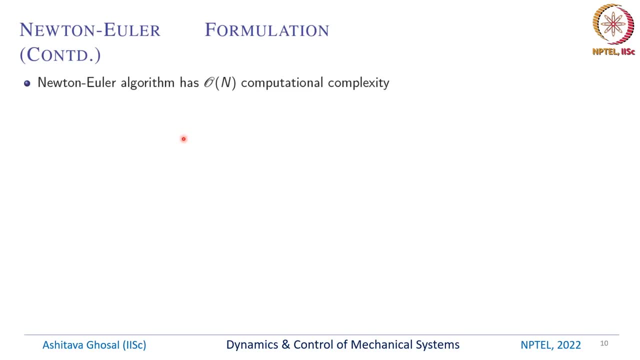 and it has been used extensively in many fields, So for example in robotics. The reason is: you can show that this Newton-Euler algorithm has O-n complexity, So this means that this is a computer science terminology, which means that the complexity increases linearly with n. 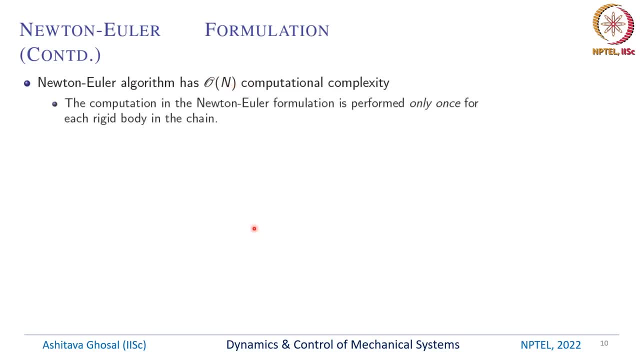 where n is the number of links. okay, So, and you can think of it this way, that the computation in the Newton-Euler formulation is performed only once for each body in the chain. So you are going outward once and then you are coming back. okay, 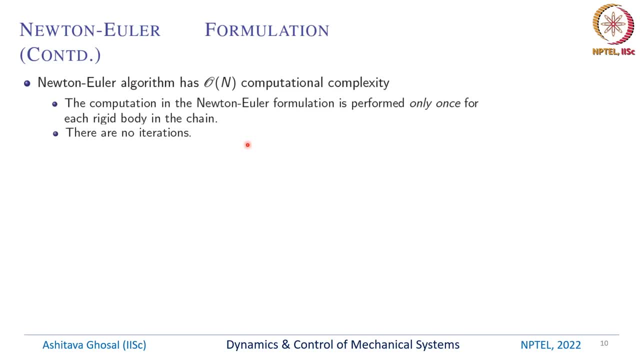 There are no loops and there is no iteration for each rigid body. If there were iterations, then it will not be linearly increasing with number of links. okay, So the number of multiplication addition is proportional to n. okay, Which n here stands? 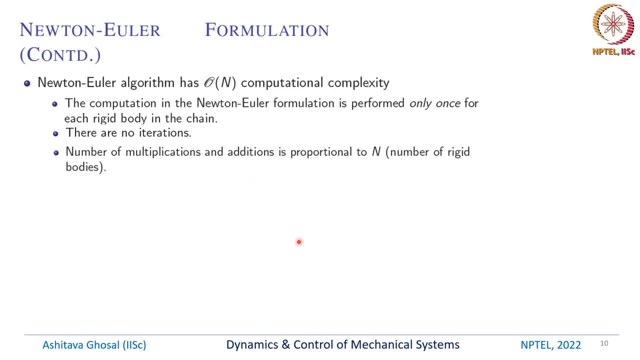 for the rigid body. have a serial chain with, let's say, six rigid bodies and you get so many multiplications and and additions. if the number of links goes to 12, then the number of multiplication and additions will become twice. okay, it will not become n square, it will not become four times, or. 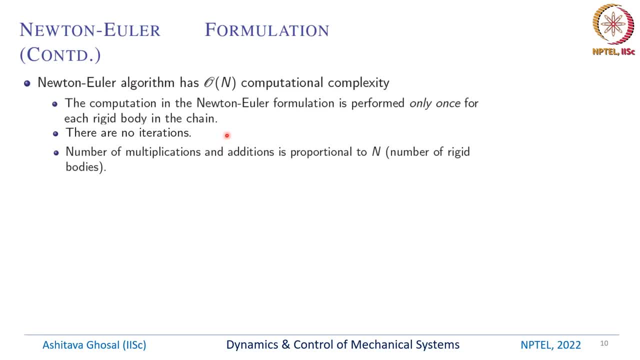 n cube. so it's a, it is linear complexity. it is very, very easily adapted for any serial chains with rotary r and prismatic joint. okay, in fact there have been extension, you can apply it for any joint. so if it was a spherical joint, if it was a three degree of freedom, spherical joint. 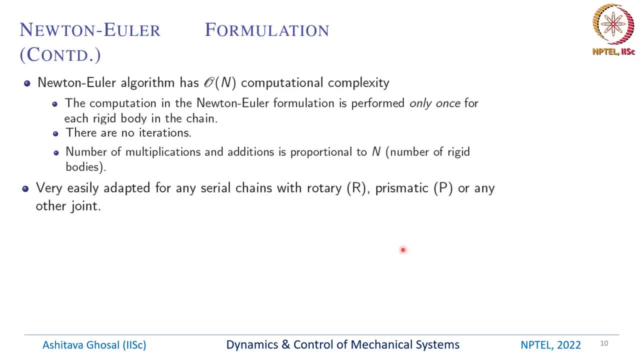 then you have to replace this spherical joint with three rotary joints. okay, but original. the newton euler formulation was mostly for rotary and prismatic joints and it can be very easily adapted to find the equations of motion for any serial chain. the other very, very useful thing in this newton euler formulation is: 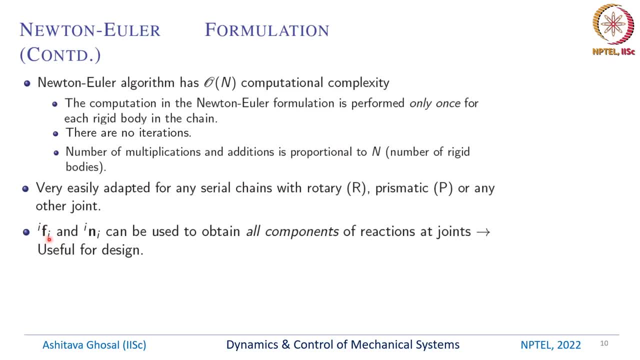 we can compute the net force, fi, and the net moment ni, which is acting at the origin of the i-th link. then we find which is the strength or tension, what is thelung'sook of this divide by the mechanism which is actually the liquidién of this neighborhood: turn92, fake state fnc. okay, so this fi has three components: fx, fy, fz. similarly, ni has three components: nx, ny and z. so the z component of n was the motor torque. but we can also find what is nx and ny. we can also find out what is fx and fy. okay, so we can find out all the components of reactions at the joints. and this is very useful. feature which we are trying to understand is whatний and what is ny. 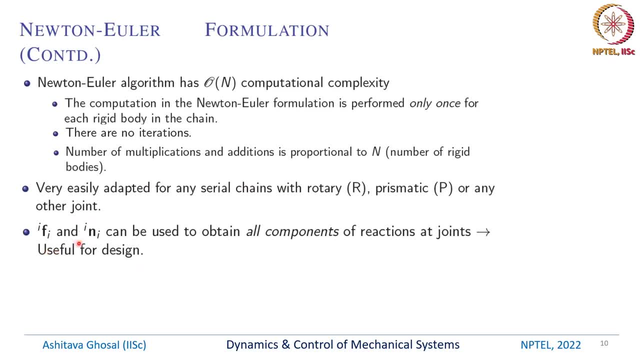 for design. So if I want to find what is the bearing which I should use for any such serial chain, I need to know all the components. I need to know Fx and Fy- okay, sometimes even Fz, or I need to know the other bearings, So then I can go about choosing what is the bearing. 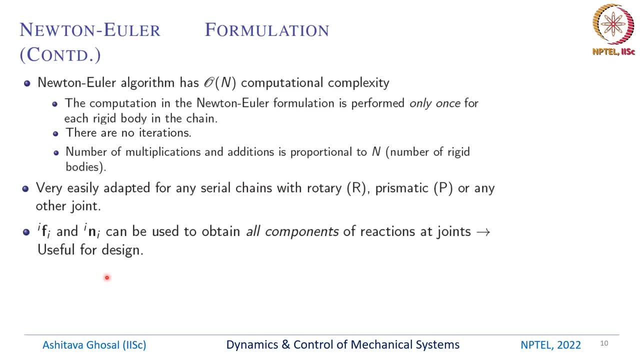 at each joint. okay, because the bearing must overcome the friction and also it can, it should, overcome the reaction forces. So we can do some kind of calculations to choose the forces which are acting at the bearing. okay, So remember, I said friction. 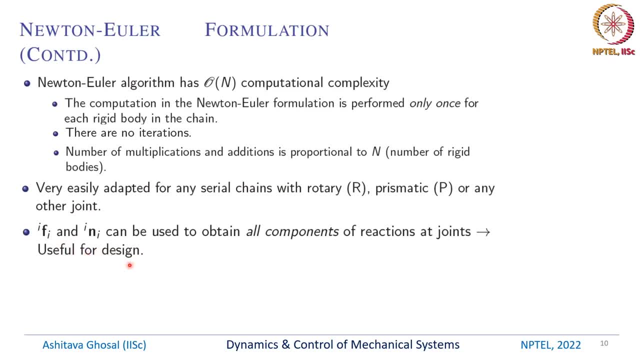 because friction also will depend on what are the reaction forces. So if there is a lot of reaction, large reaction, then the friction might be more. The other very nice feature of this Newton-Euler formulation is it is very easy to use. So if you have a lot of reaction you can use a lot of reaction. 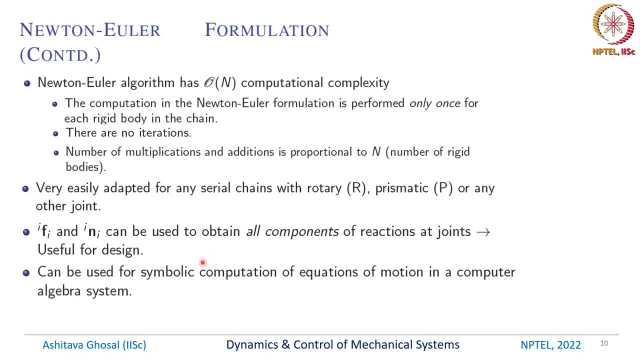 very, very mechanical, okay, So you go from position velocity acceleration for one link, then you go to the next link, and so on, and then at the end of position velocity acceleration, you calculate the F, which is Ma, and N, which is I. alpha plus omega, cross I omega We use. 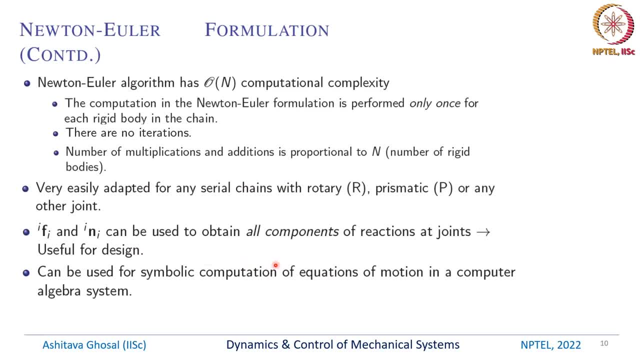 Newton's law and Euler's equation and then we go backwards and we find what are the joint torques of the joint forces. So we can use the Newton-Euler equation and then we go backwards and we find what are the joint torques of the joint forces. So this is very, very mechanical and it can be. 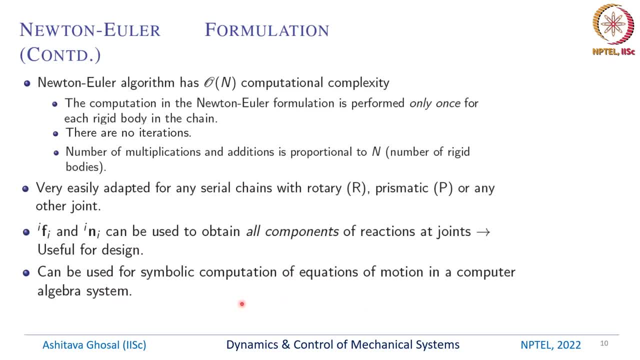 easily done, you know, by symbolic computation. We don't need to sit down and work all these steps by hand. In fact, there are computer algebra systems, and I will show you one which is called Maple, which can be very easily used to compute all the steps one by one, symbolically, not using 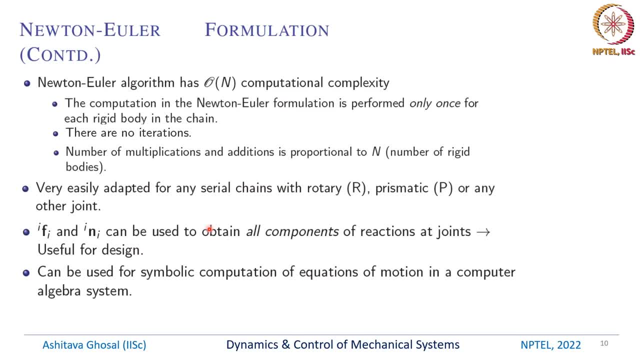 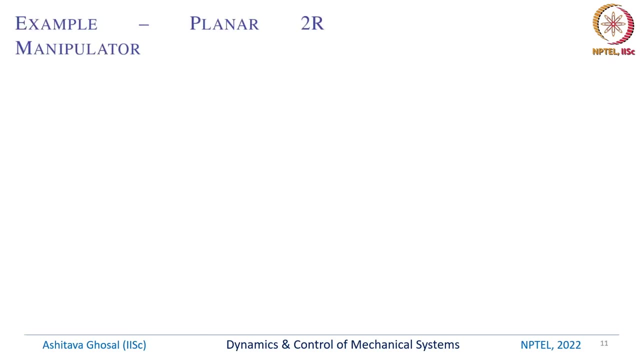 numbers And eventually we can end up with the equations of the Newton-Euler equation. So this is the equation of motion and it is extensively used in robotics. It is extensively used in many other places which have serial chains. So let's look at an example. So we will take our simplest. 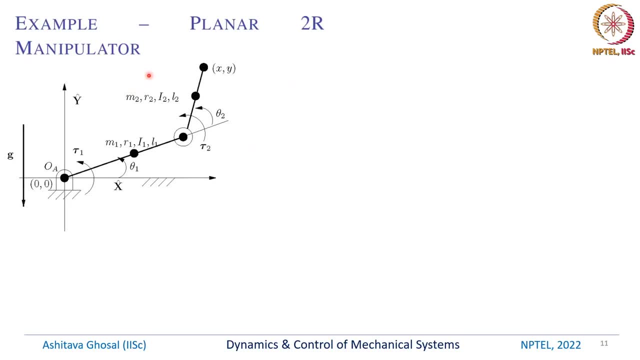 possible example of a planar 2R manipulator. Remember, we had worked out the equations of motion using very basic mechanics, which was Newton's law and Euler's equation, So we can look at some of the external moment was I times, alpha and so on. And then we, you know, we could 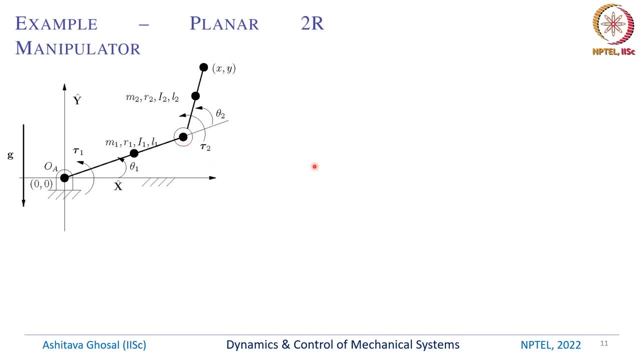 eliminate the reaction forces at these joints and then we derive the equations of motion. Now I want to take the same example and go through the steps of this Newton-Euler formulation and I will show you, obviously, that the equations of motion are same. 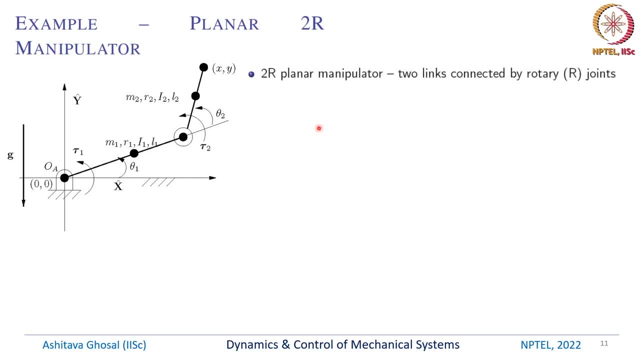 So what do we have? We have two degrees of freedom, We have two links and there are two rotary joints. So this is the fixed base with 0, 0. This is the origin of the fixed coordinate system x and y. Then we have one link and again theta 1 and theta 2 are the rotations. 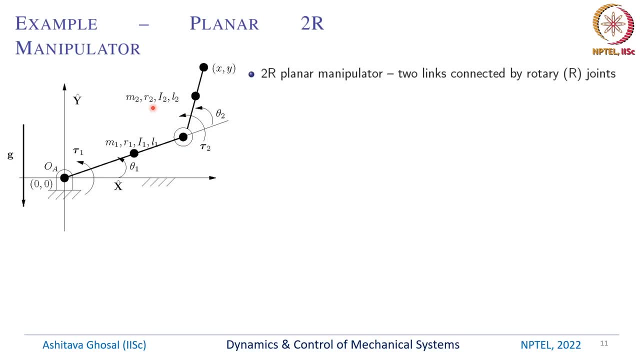 the rotary joints And, just like before, we have: m2 is the mass of second link. r2 is the location of the cg, So this is the mass of second link. r2 is the location of the cg, So this is the. 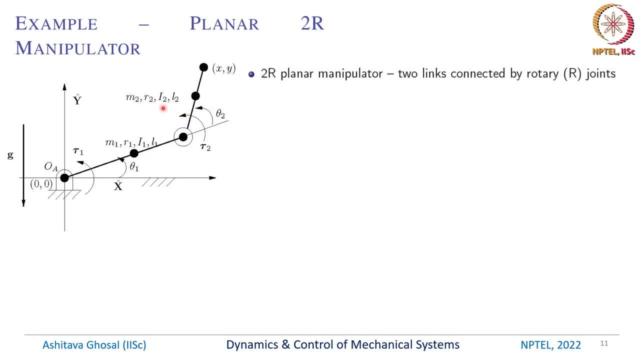 I2 is the z component of the inertia matrix, L2 is this length, and so on. Okay, So, for rigid body 1, we have m1, r1, I1, which is the z component, and L1.. And for rigid body 2, which is m2, r2,. 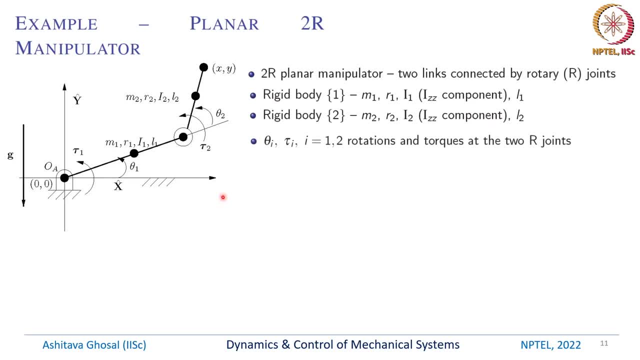 I2, and L2.. Theta is the rotation of the first one. two joints, theta 1 and theta 2, and tau y I equals 1 and 2, are the torques which are being given by this, at these joints by motors. 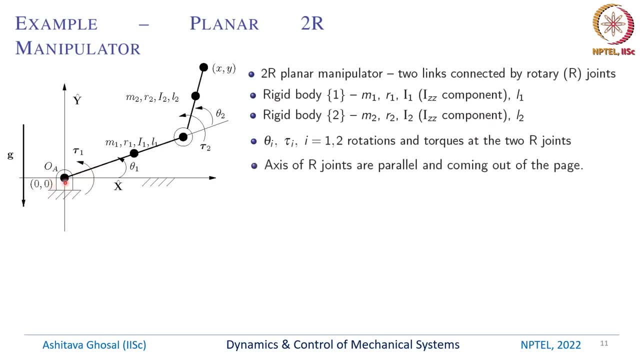 let's say The axis of these r joints, which is here and here they are parallel and they're coming out of the page. So this is the z axis, This is x, y and, if you use the right-hand rule, 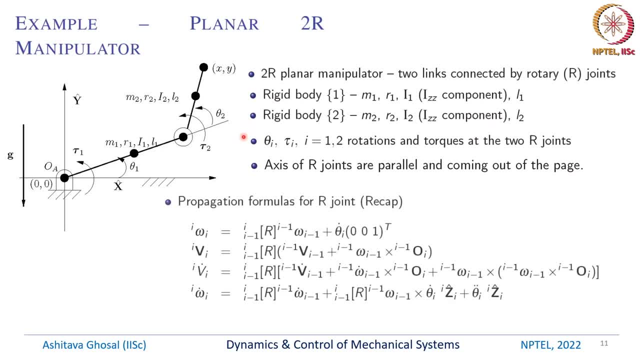 the z axis is coming towards you. So let's do the recap of the propagation modulus. So we have: angular velocity of the ith link is related to the angular velocity of the I minus 1th link plus some theta dot. Similarly, linear velocity of the ith link, which means: 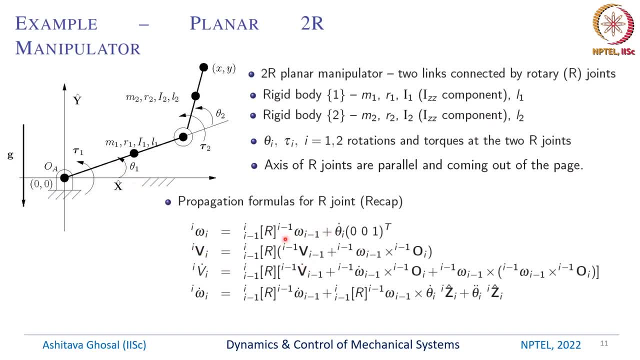 linear velocity of the origin of the ith link is nothing but the linear velocity of the I minus 1th link plus omega cross r. The acceleration is similarly acceleration of the origin Plus alpha times r plus omega cross, omega cross r And angular acceleration is the angular. 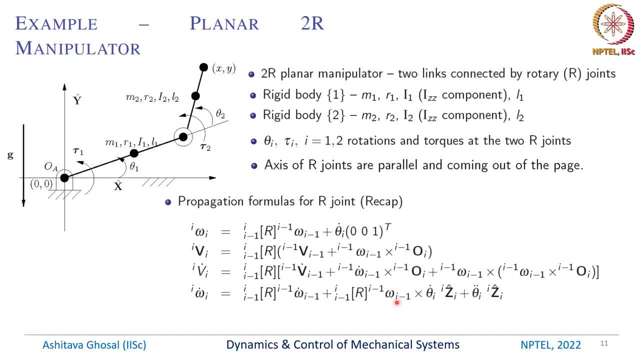 acceleration of the previous link, plus this omega cross, theta dot and then theta double dot along the z axis. So these are the four propagation equations which we will use, And we also have the acceleration of the center of mass of each link, which is nothing. 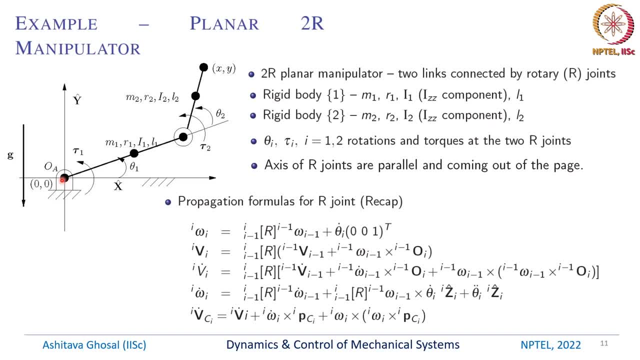 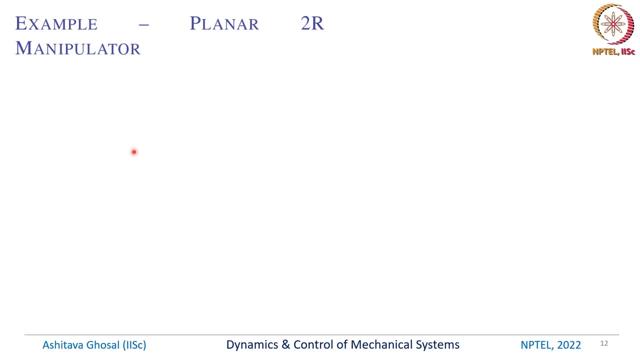 but the acceleration of the origin of the link: plus omega cross r plus alpha times r. Sorry, omega cross, omega cross r plus alpha times r. So let us continue. We have this 2r planar, 2r manipulator. Zero is the fixed. 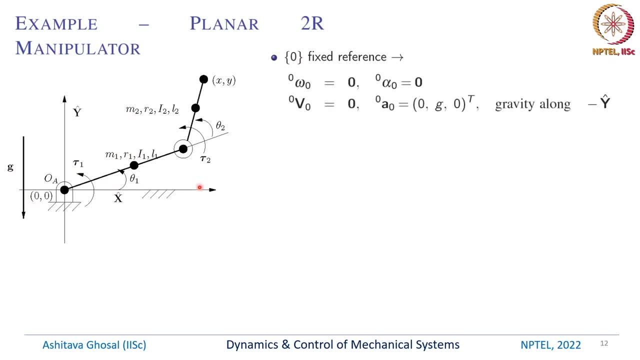 reference, And if you have zero as the fixed reference, nothing is moving. So the angular velocity of the 0th coordinate system is zero, Angular acceleration is zero, The linear velocity of the origin of the 0th coordinate system, which is this point, is zero, And the acceleration of 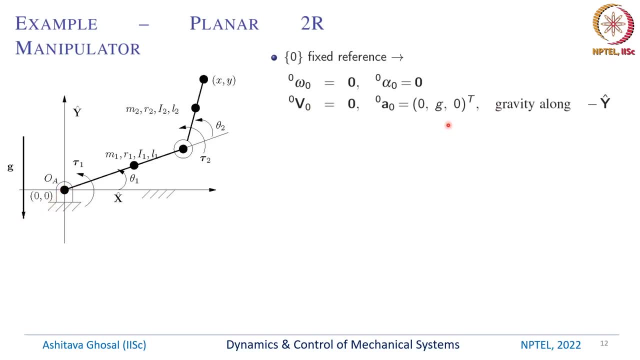 the origin of the 0th coordinate system is g. Remember, we want to also capture the effect of gravity And if you want to capture the effect of gravity, you have to capture the effect of gravity. We have this base accelerating upwards by g. g here is 9.81 meters per second And it is along 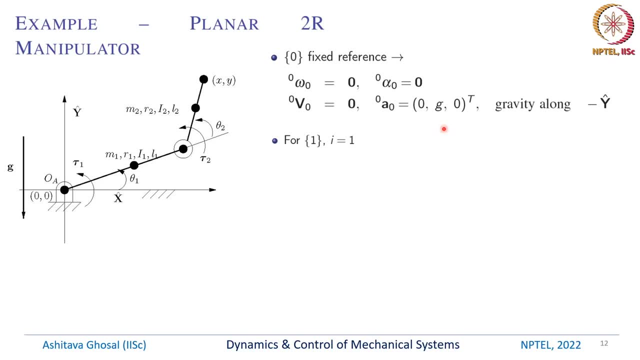 the y axis. So for i equals 1,. we use this propagation formulas, which was i1. omega 1 will give me 0, 0, theta 1, dot 1, b1 will be zero, 1, a1 will still be zero, 1, alpha 1,. 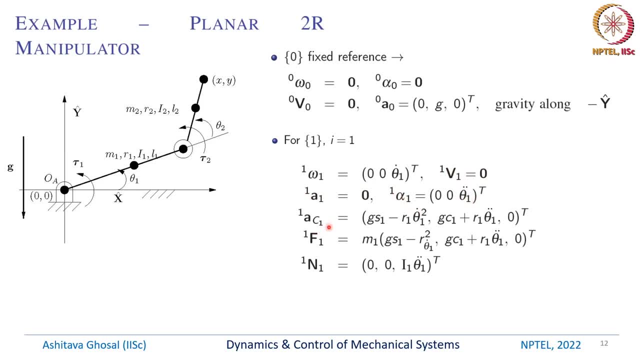 is 0, 0, theta 1 double dot. The acceleration of the center of mass of the first link is gs1 minus r1, theta 1 dot square. The y component is gc1 plus r1, theta 1 double dot 0.. Here we can see. 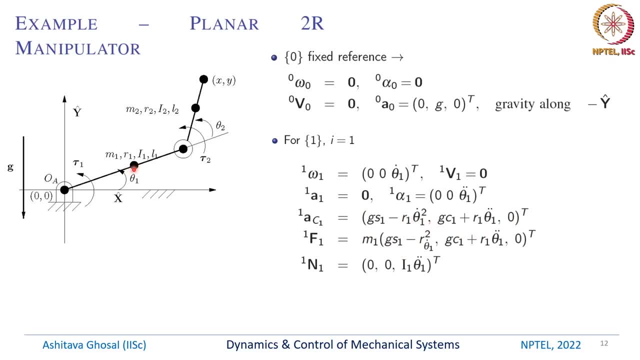 that it looks okay, right That the center of mass here, which is here, there will be a Coriolis term which is r1 theta 1 dot square, which is going towards, And then there will be a tangential term which is r1 theta 1 double dot, And then, of course, we have g. 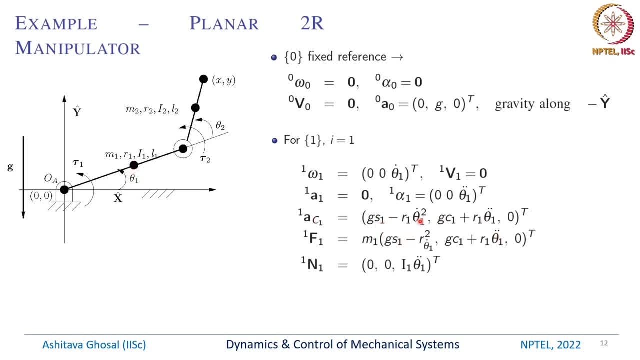 which is coming down. But now we have this sine theta 1 and cos theta 1, okay, Because we are rewriting all these terms. in its own coordinate system, The Newton's law tells me that the force f1 will be mass times this acceleration, And that is exactly what is written here. So we take this. 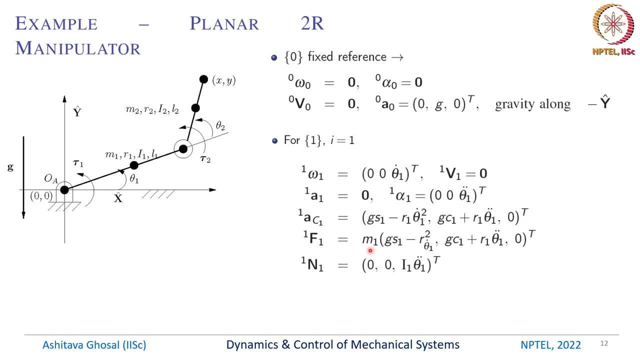 acceleration vector and multiply by m1.. Euler's equation tells me that the moment, external moment, is nothing. but i times theta, 1, double dot, i times alpha, Because remember, omega cross i, omega is again zero. So let's continue. So for i equals 2, for second link we substitute: 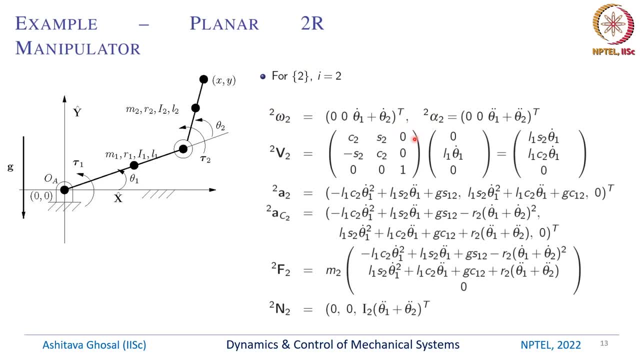 what is 1 omega 1, 1 v 1, 1 alpha 1, and so on in this propagation equation? And we can find: 2 omega 2 is 0,, 0 theta 1 dot plus theta 2 dot. okay, That makes sense, right? That the angular velocity of 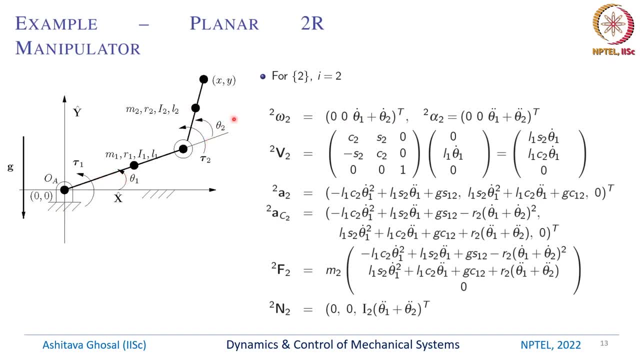 the second link will be the sum of theta 1 dot and theta 2 dot. Theta 2 is relative rotation, So the angular velocities will be summation Of theta 1 dot and theta 2 dot. The acceleration is derivative of this, So we'll get theta 1 double. 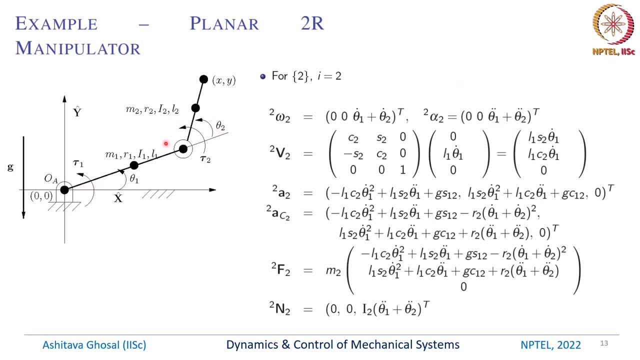 dot plus theta 2 double dot. The linear velocity, okay, of the origin of this second link, which is basically this term, will be some matrix times 0: l1 theta dot 0.. So where is this l1 theta 1 dot? 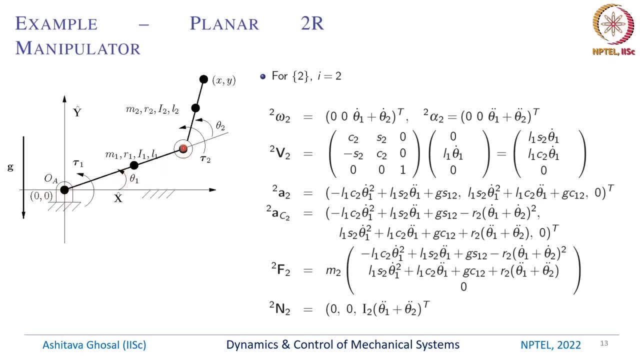 coming from. So this is l1.. There's a theta 1 dot here, So there is a velocity component in this. So this is the local y, this is the local x direction, this is the local y direction. so that's why we have zero l1 theta. 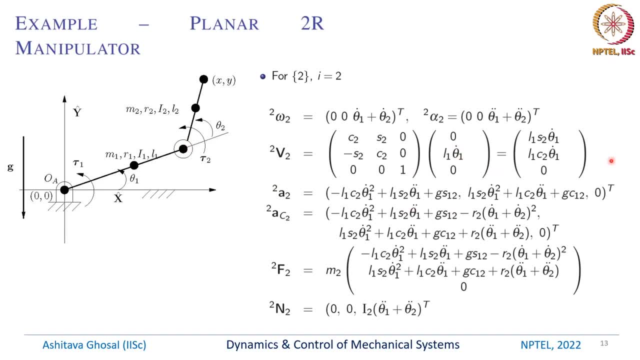 1 dot, and then we pre-multiply by a rotation matrix, so hence the linear velocity of this origin of the second link, written in its own coordinate system, is: l1 s2- theta 1 dot. l1 c2 theta 1 dot zero. okay, so there is nothing very confusing about this whole thing, except that we 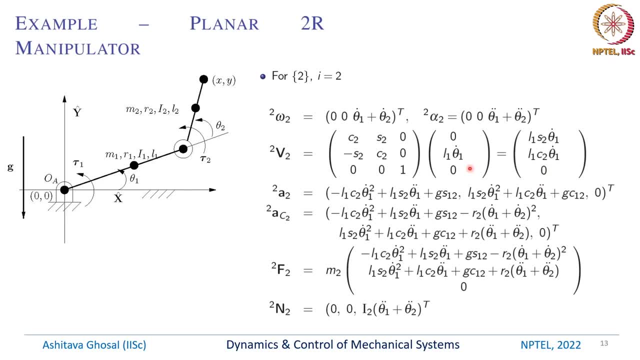 are mechanically using those propagation equations. so if you write down the propagation equation on a sheet of paper and then you just substitute, you will get these terms. likewise, the acceleration of the origin of the second link will have three terms. okay, there will be a gravity then there. 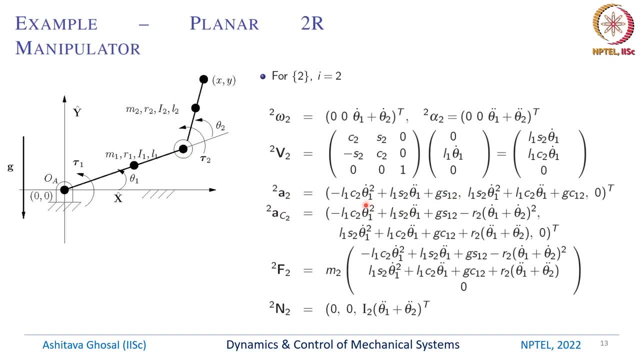 will be a theta one double dot and there will be a theta 1 dot square. okay, that is what you will get. this is the origin of this point. so this one. there will be a theta 1 double dot, which is this direction: theta 1 dot square, which is this: 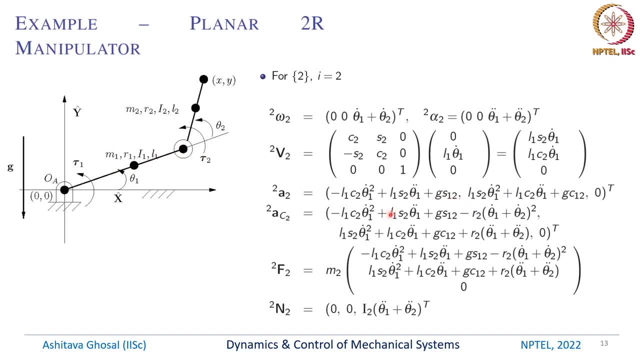 direction. and then there is this gravity term. similarly for y component we'll have theta 1 dot, square one term with theta 1 double dot, and again gravity. the z component in all these expressions are zero, both velocity as well as acceleration, because this is a planar system. 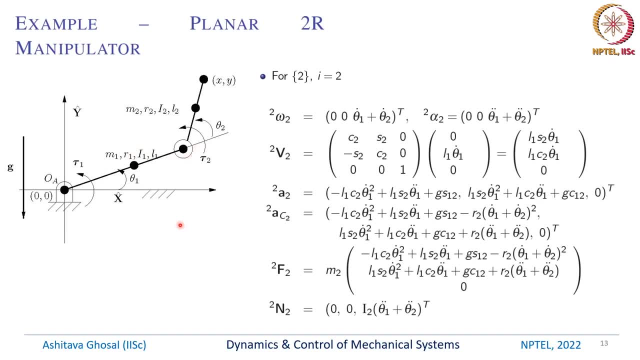 all the motion is happening in the x- y plane. the cg of this second link is at a distance r2 from here. okay, so what? the acceleration of the cg will be nothing but the acceleration of this plus some effect of this r2. okay, so that is what you get. so you will get some term which is r2. 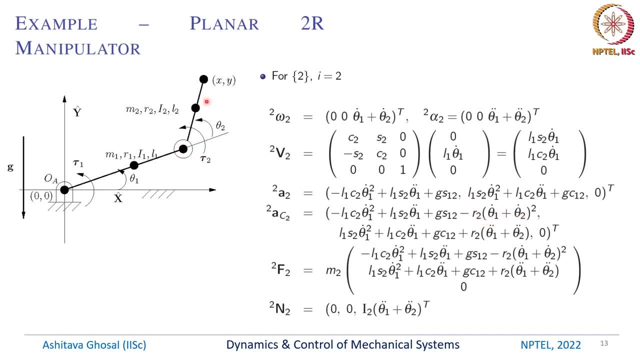 theta 1 dot plus theta 2 dot, whole square. and then of course we'll have some l1 s2- theta 1 dot and l1 c2- theta 1 dot square, and so on. so theta 1 dot square- this term is coming from here- gs2. 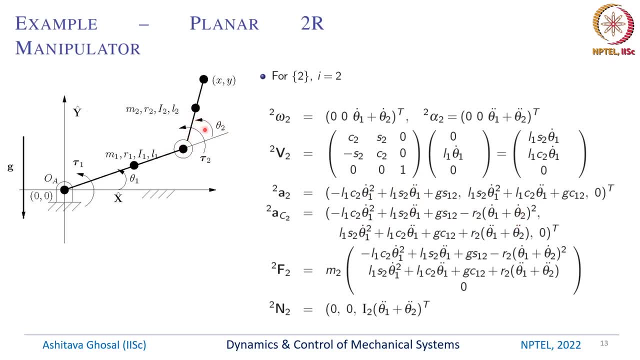 is coming from here. but then we have this centripetal term, which is coming because the center of mass is at a distance r2 from the origin of the second link. okay, so we can find this acceleration of the cg of the second link, and then we apply euler's equation. 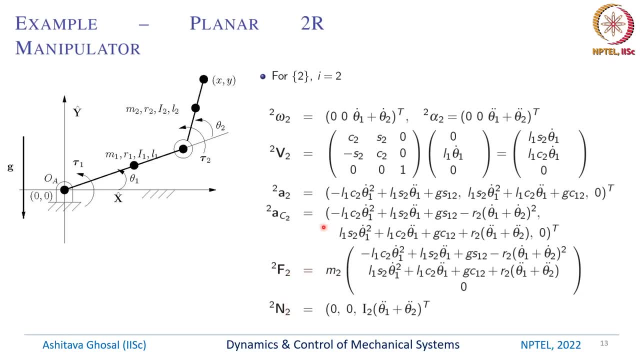 and Newton's law. Newton's law says that the force is nothing but m2 times ac2, which is what is written here. so it is m2 times this vector. so you can see: the first term is minus l1 c2, theta 1 dot square. here also it is minus l1 c2, theta 1 dot square. so this is just the x component. so m2 is the moment of mach. 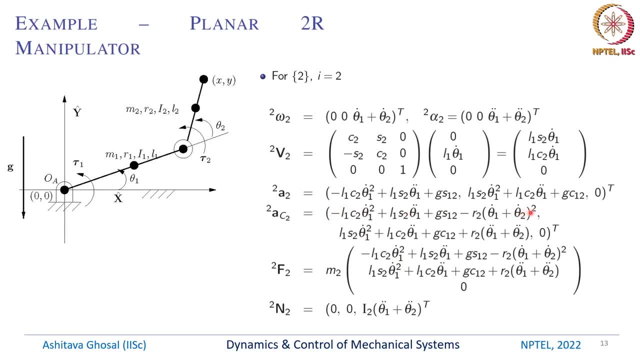 完全在 tricka sounded: x component, so m2 into the x component, m2 into the y component and again zero. and Euler equation tells me that this is I2 into theta 1 double dot plus theta 2 double dot. okay, so this, these are the. 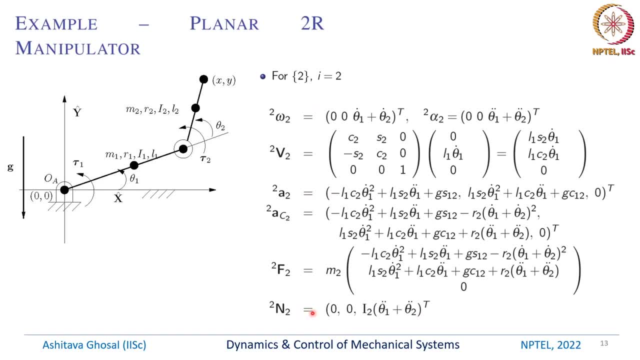 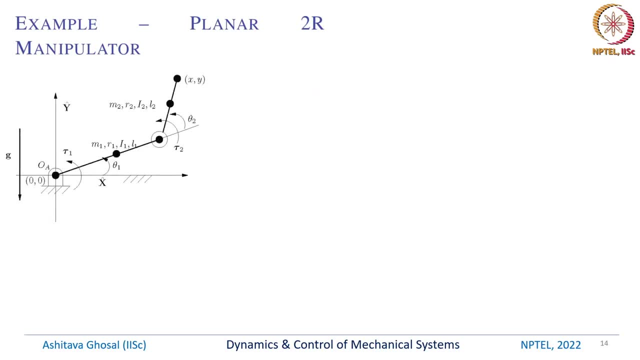 equations for I equals 2, we have also found out what is for I equals 1, which is the link 1, and then we go back and do this inward propagation of forces and moments. so we want to compute the joint torques which is happening, this tau 1 and tau 2, so basically we have this force which is 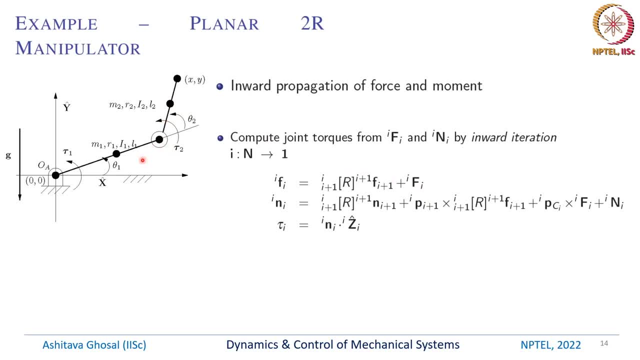 acting here, which is fi, and then we have this external force. in this case, maybe zero, there is no external force happening acting on this link, but if there were any, we have to add that here, and then we have this external force acting on this link, and then we have this external force. 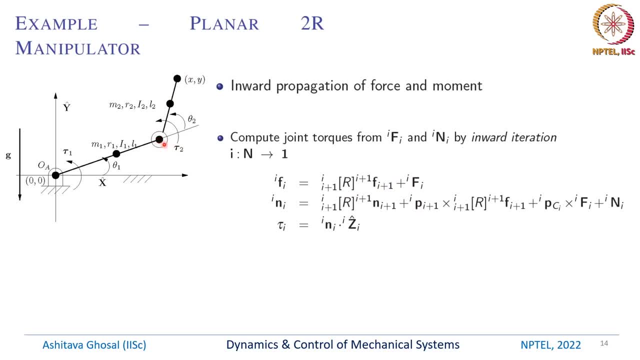 acting on this link, and then we have this external force acting on this link, and then we have this, And that gives me what is the force acting at the origin of the ith coordinate system, What is the moment which is acting at the origin of the ith coordinate system? 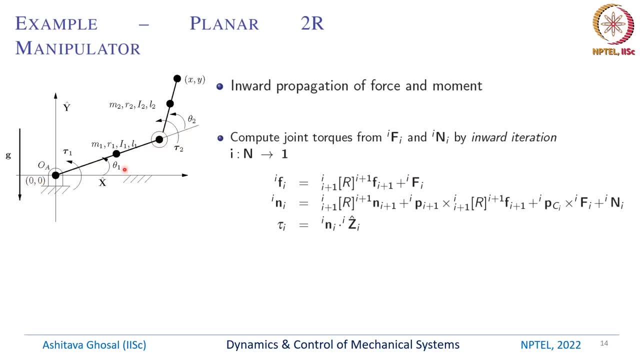 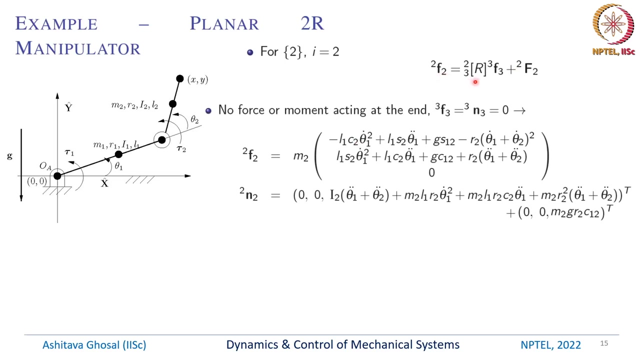 And the torque. in this case, since they are rotary joints, both of them we will get. the z component of the moment is resisted by this motor, or this motor is giving the equivalent of the z component of the moment. Okay, so for I equals 2, we have, 2F2 is nothing but 2, 3R, 3F3,, 2F2.. 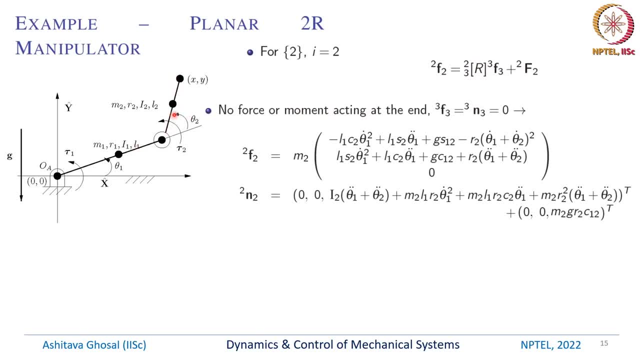 So there are no forces which are acting on the third link in this example. If there are force and a moment- external force and moment- which is acting on this link, then we have to take those into account here. So these two are zero. 2F2 is nothing but this. 2F2 is nothing but capital F2.. 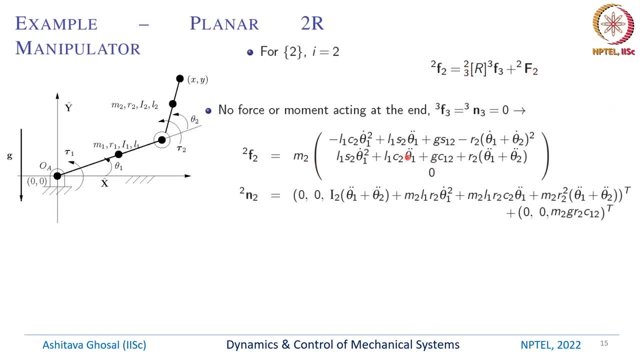 Which is mass times the acceleration, And 2N2 is nothing but the I times alpha, whatever you will get these terms. Okay, so I2 into theta 1 double dot plus theta 2 double dot plus M2L1R2, theta 1 dot square, and so on. 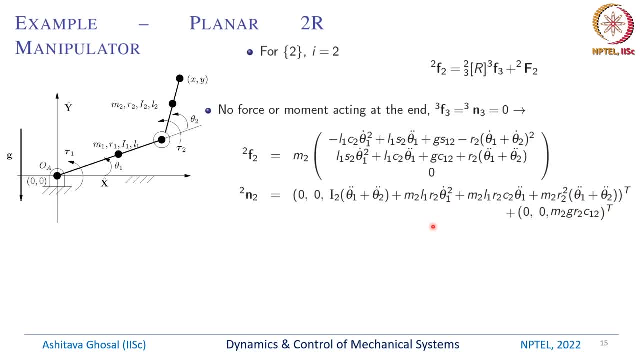 Okay, so this is like the alpha and the omega part. Okay, So the torque at joint 2 is nothing but the z component of N2.. So this is 2N2 dot product with 001, which is the z component, And hence we will get this last 1,, 2,, 3, 4 terms. 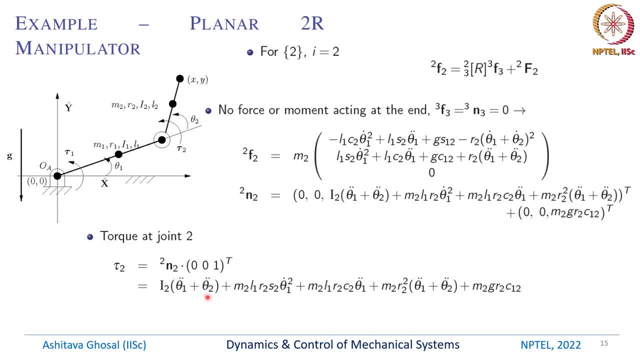 So tau 2 is I2 into theta 1 double dot plus theta 2 double dot plus M2L1R2S2 theta 1 dot square plus M2L1R2C2 theta 1 double dot plus M2R2S2 theta 1 dot square plus M2L1R2C2 theta 1 double dot plus M2R2C2 theta 1 double dot algorithms. 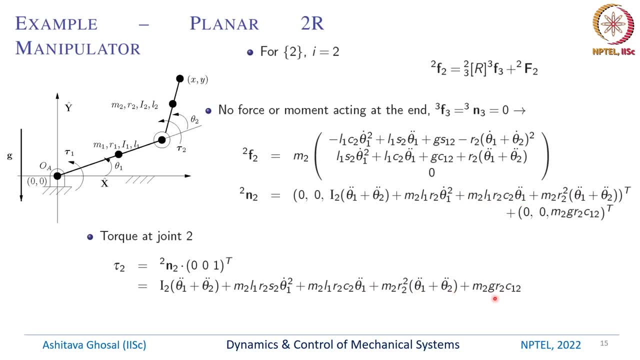 r2 square, theta 1 double dot plus theta 2 double dot and then this gravity term which is m2, g, r2, c12. okay, so this is the equation of motion, for the one of the two equations of motion, which is tau 2, is given by some i into theta double dot plus some Coriolis term and some gravity term. 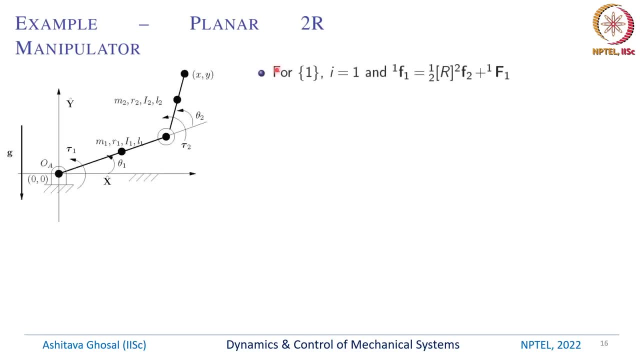 so likewise, for i equals 1, we have 1. f1 is nothing but 1 capital f1 plus this 2 f2, so inward propagation. so the force which is acting at the origin of the second link will be seen at the origin of the first link, which is this: 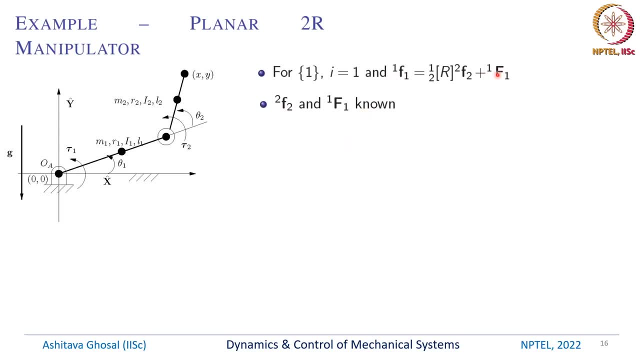 okay. and then 2 f2 and 1- f1 is known from the previous step. so the moment which is acting at the origin of the second link will be seen at the origin of the second link, at the origin of the first link is given by the. this is from euler's equation. this is the moment. 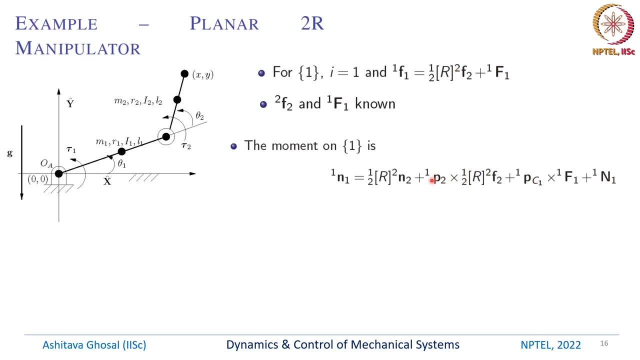 of this force, f1, and these are the force which are coming from the second link to the first link. okay, so hence the joint torque is nothing but one n, one dot, zero, zero, one. so we know what is 2f2, we know what is 1f1, we know what is 1n1 from euler's equation. then we substitute everything. 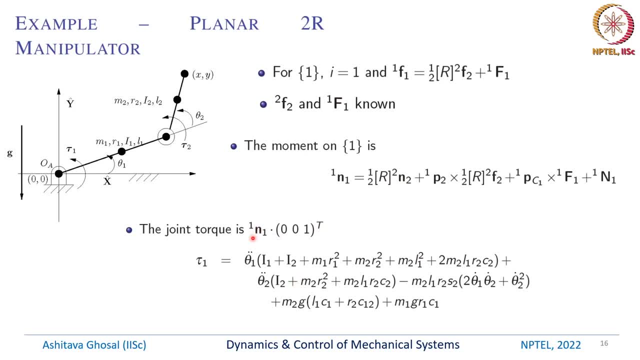 here and then we take this z component of 1 and 1 and you will get tau 1 is given by this. okay, so this is the second equation for this planar 2r manipulator. so the first equation said tau 2 will was something now we have. tau 1 is equal to theta 1 dot. 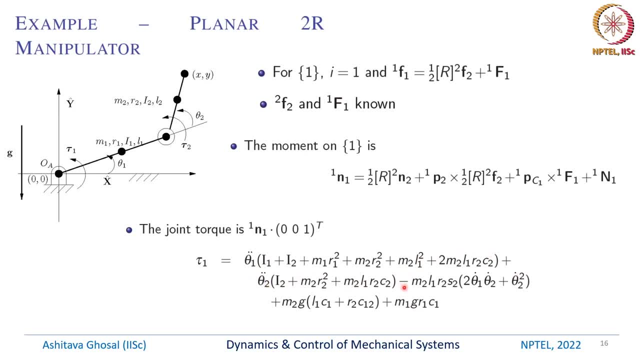 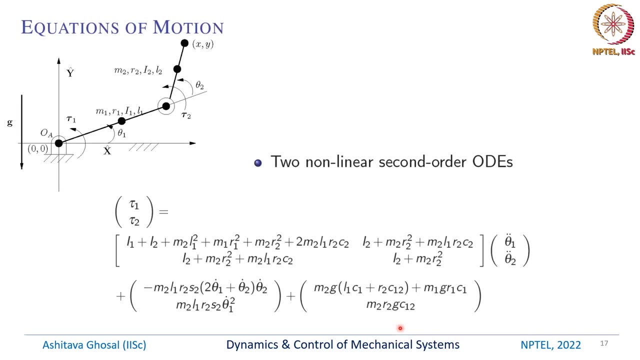 double dot into some terms here, theta 2 double dot into some terms here, and then we have this: 2 theta 1 dot, theta 2 dot, theta 2 dot, square, and then some gravity term. okay, so what do we have finally for this two link system, two serial, two links connected serially by rotary joints. we have two non-linear. 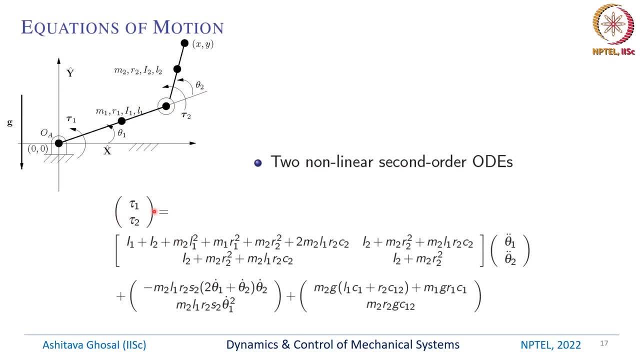 second-order odes. and these second-order odes are that we have tau 1 is something into theta 1 double dot, plus something into theta 2 double dot, plus some terms which are theta 1 dot, theta 2 dot, theta 2 dot square, and some term which is gravity, which is g into l 1 cos theta 1 r. 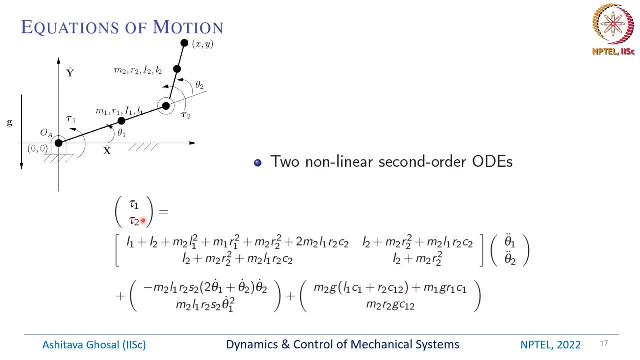 2 cos theta 1 plus 2, and so on. likewise we have a term equation which is: tau 2 equals I2 plus m2 r2. square into m2 l1, r2 c2 into theta 1. double dot plus I2 plus m2 r2, square into: 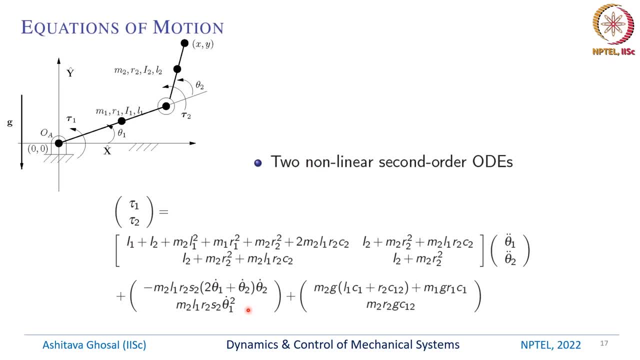 theta 2 double dot, plus a term which is theta 1 dot, square into something, and one term which is gravity term. okay, so we have these two second order equations written in this vector and matrix form. so tau 1 and tau 2 is a 2 by 1 vector. this is a 2 by 2 matrix multiplying theta 1 double dot. 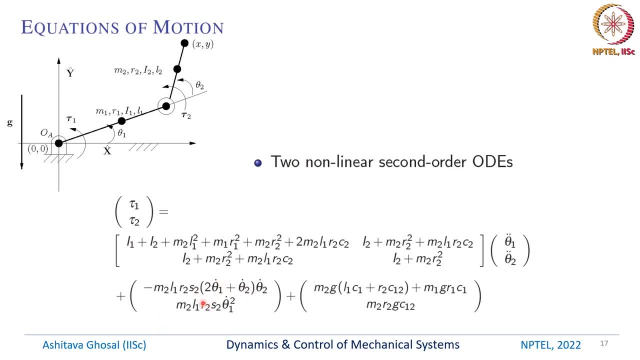 theta 2 double dot. then we have this vector, two components, one which is 2 theta 1 dot into theta 2 dot, into something, and then theta 2 dot square. and remember, all these are multiplied by some sine theta 2. here is there some cos theta 1 plus 2 here, and this is cos theta 2. 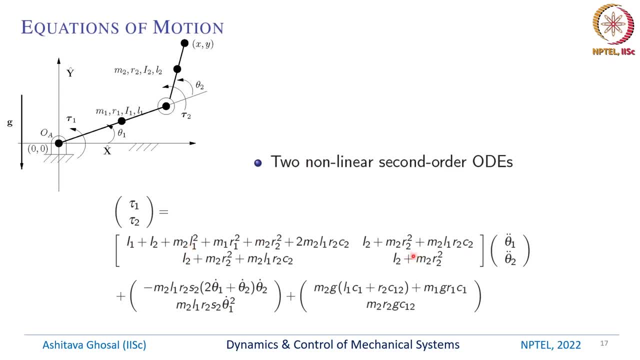 so? So the elements of this matrix are not constant. They are dependent on theta 1 and theta 2.. So this term here, if this theta 2 is 30 degrees, you will get something, but if it is some other, 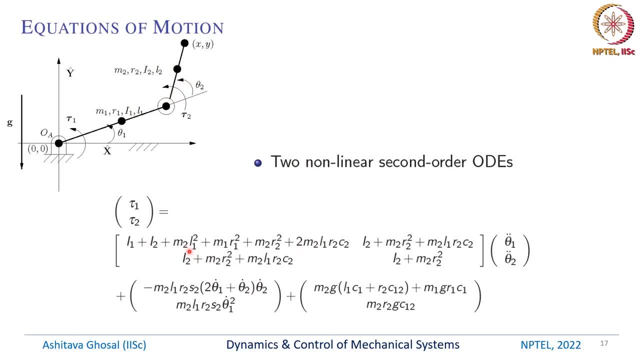 angle. you will get some other terms here: I1, I2, M2, L1, R1, these are all constant but theta 2 is changing. So if theta 2 is changing the elements of this 2 by 2 matrices. 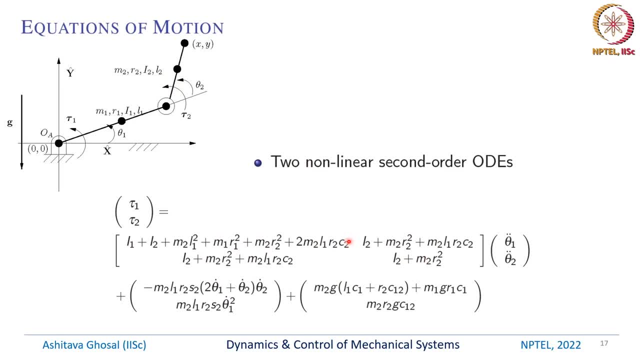 are changing and which is why it is a nonlinear second order ODE. So the coefficients of theta 1 double dot and theta 2 double dot are not constant. Some are constant. So for example, in the second equation, this is I2 plus M2, R2 square into theta 2 double dot. So 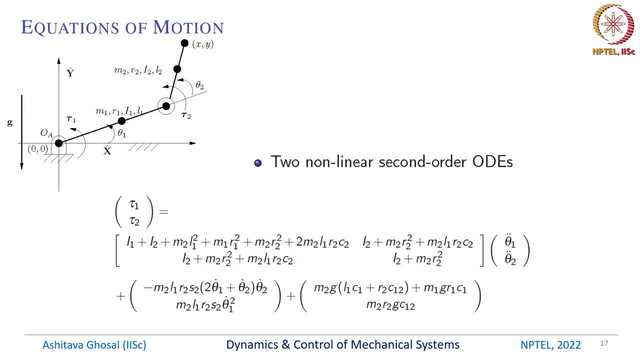 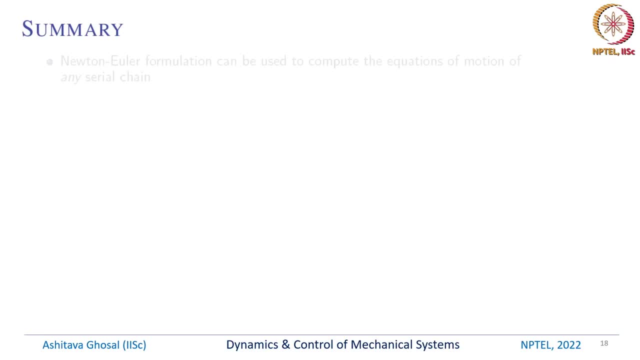 this is constant, but this other term has cosine theta 2.. And the equations of motion that you have got are exactly same as what we had got earlier using hand calculations, when we did not use these propagation formulas. So, in summary, the Newton-Euler formulation can be used to compute the equations of motion of 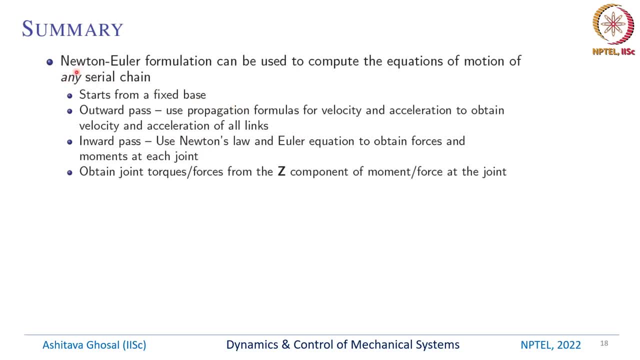 any serial chain. This is an important word. So if you give me a serial chain with five links, yes, If you give me one with 100 links, again I can find out the equations of motion. Of course, for a 100 link you will have huge, 100 such second order ODEs. So we start from a fixed base. 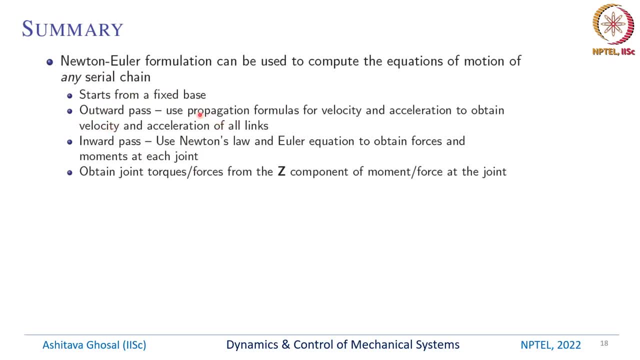 We do an outward pass. The outward pass consists of propagation formulas for velocity and acceleration to obtain velocity and acceleration of all links. And then there is an inward pass. We use Newton's law and Euler's equation. So we have to take the force of the moment at the joint to obtain forces and moments at each joint. 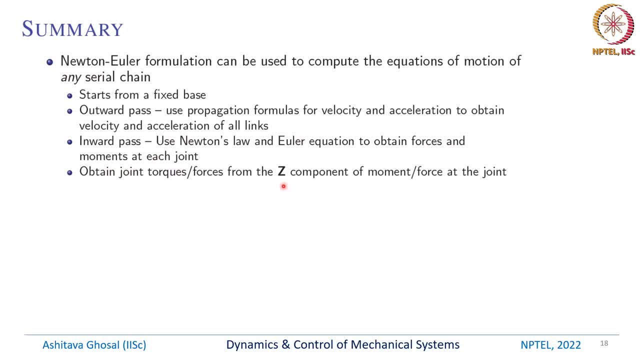 And then we obtain the joint torques or forces from the Z component of the moment or force at the joint. Okay, So in the examples which I showed you, it was the Z component of Ni Ni was the moment, But if it was a prismatic joint, then we have to take the Z component of Fi. 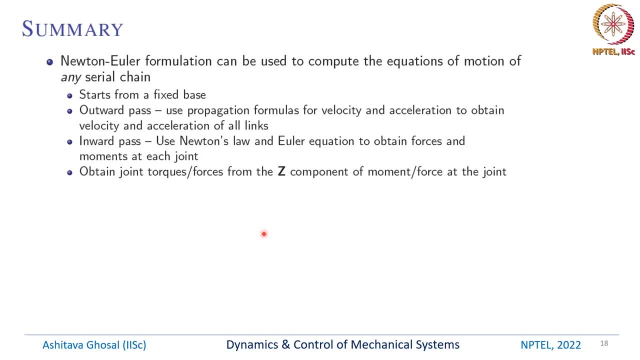 which is the force which is acting on the origin of the ith link. This is a very, very efficient algorithm. It is as I said. it has O-N complexity. It is linear in complexity. So if the number of links becomes double, the number of additions. 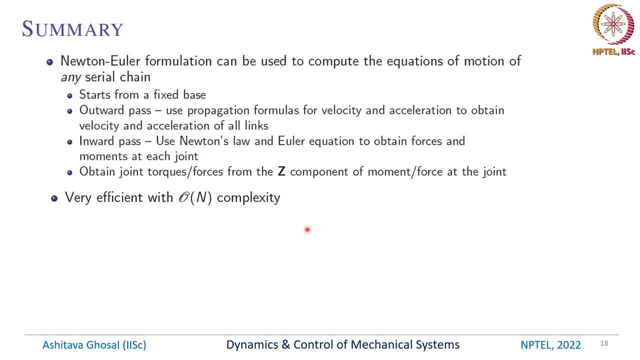 and multiplications and the complexity also scales by 2. It does not scale by 2 square, or even there are some algorithms which can be exponential complexity, So the number of N is increased by twice. It will be some to the power of N cube or, you know, it could be N. 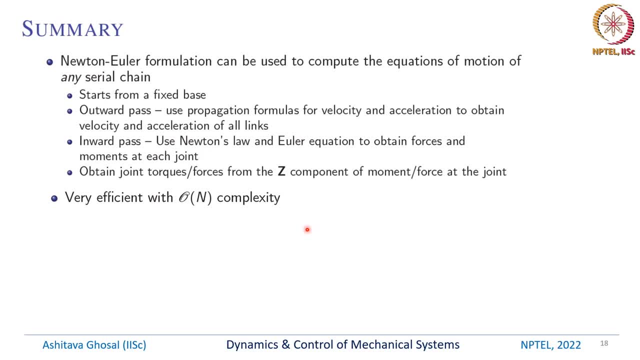 square or E to the power N. So that is not what is happening here. This scales linearly. The unfortunate part is it is not very easily applicable for parallel structures. It is very, very efficient for serial chain, but not really applicable for parallel structures. 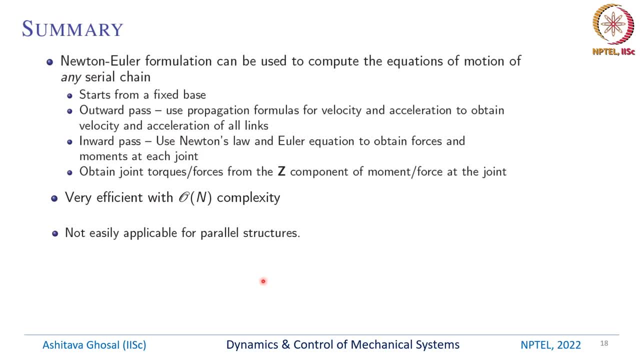 So the basic problem with parallel structures, which you have seen, is that there are loops, So I can start from one fixed end and I can come back to the fixed end again. Okay, So hence we cannot go outwards till one last link and come back. That is not possible. 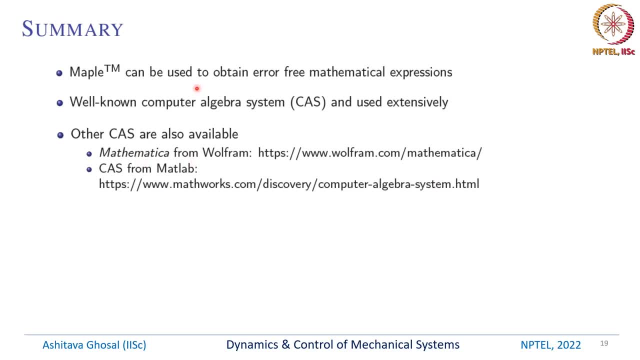 So, in summary, Maple can be used to obtain error-free mathematical expressions. So I can find out the elements of the mass matrix, the elements of the Coriolis term, the elements of the gravity term, the elements of the constraint matrix, the derivative of the constraint matrix. 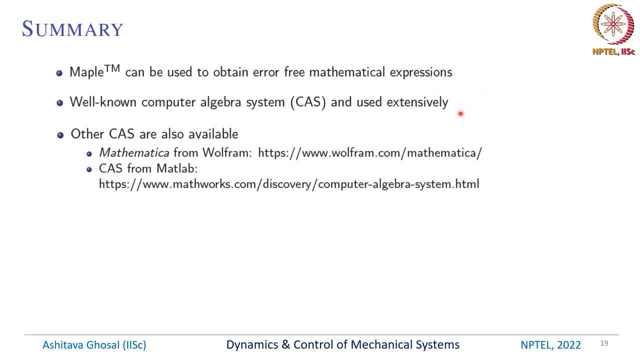 and so on. Then we can form the equations of motion and solve the equations of motion in MATLAB or some other, you know, software which allows you to use numerical numbers or numerical tools, like ODE solvers and so on, which can solve these differential equations of motion. 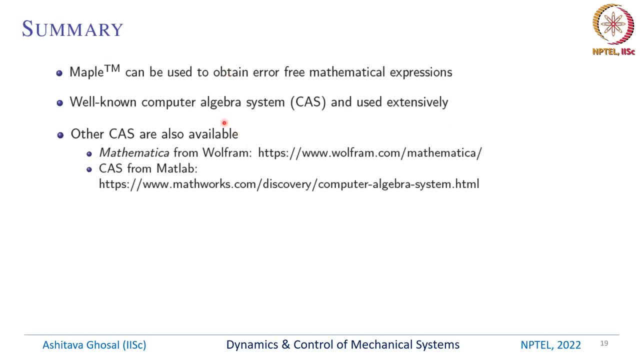 So what I have showed you is one of the computer algebra system which is well-known: Maple. It is used reasonably extensively. There are other computer algebra systems which are also available. There is another very well-known CIS system which is called Mathematica It.